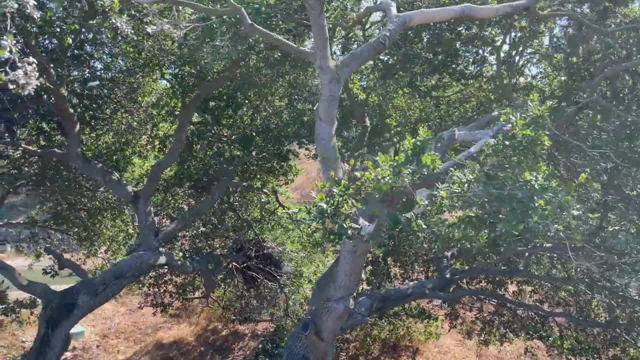 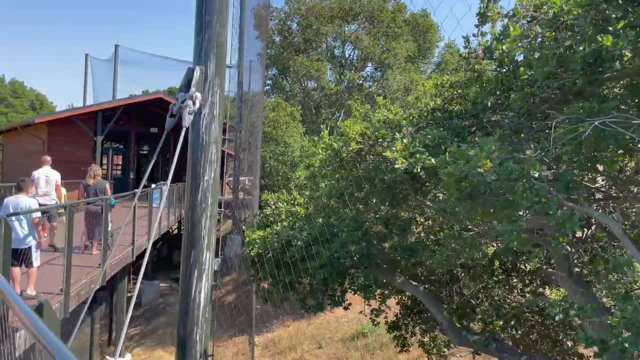 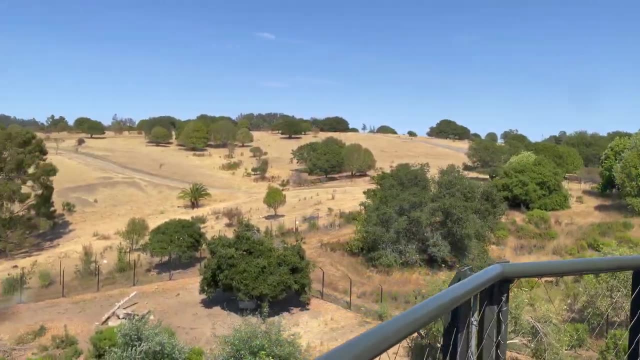 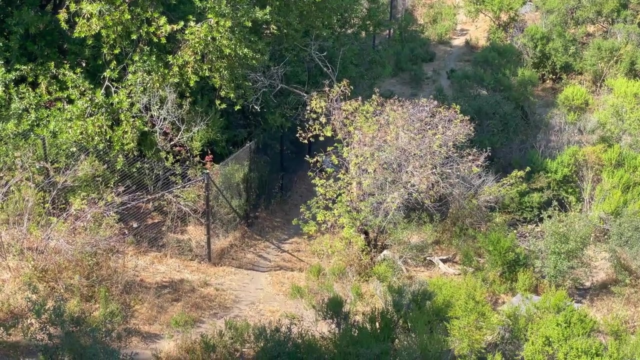 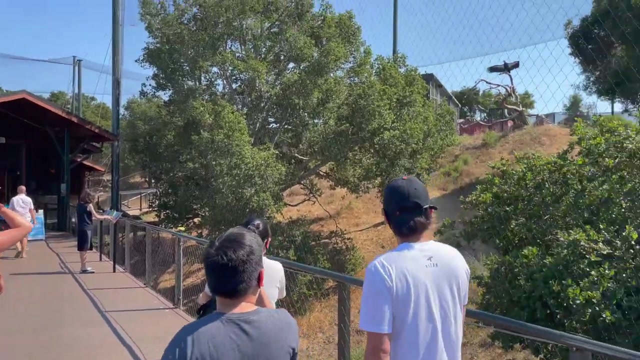 Thank you, Nice to meet you. Look, you guys Sit over here. Where is it? Look at this coyote, A wolf Junior. come here. I think it's right there sleeping by the fence. Oh, no, no, oh, look at the things. 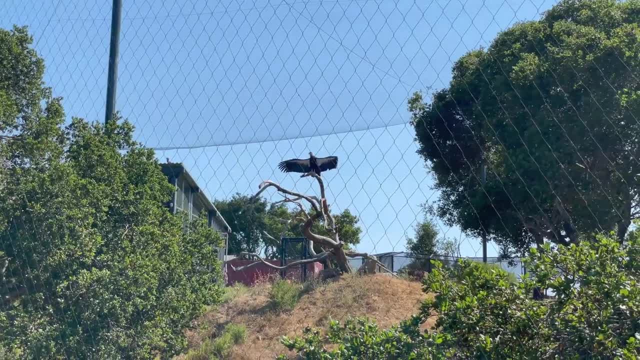 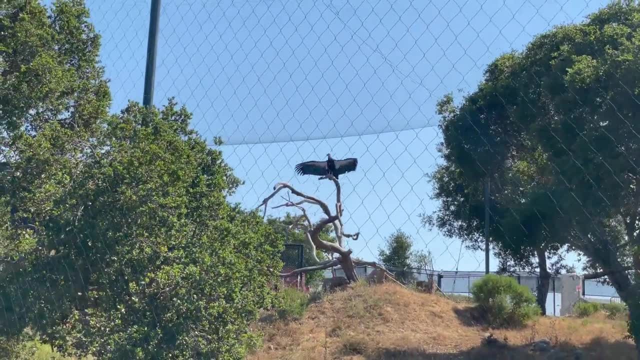 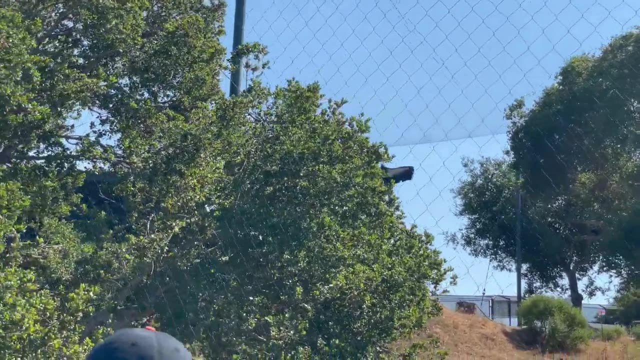 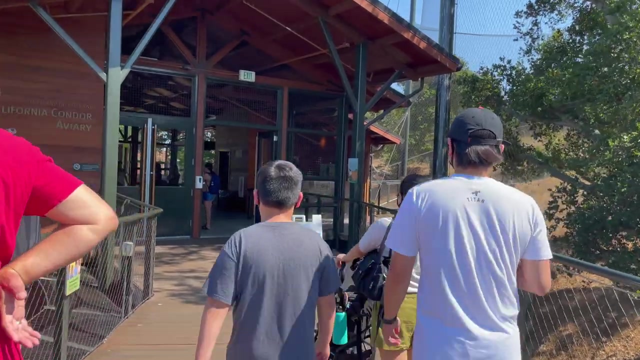 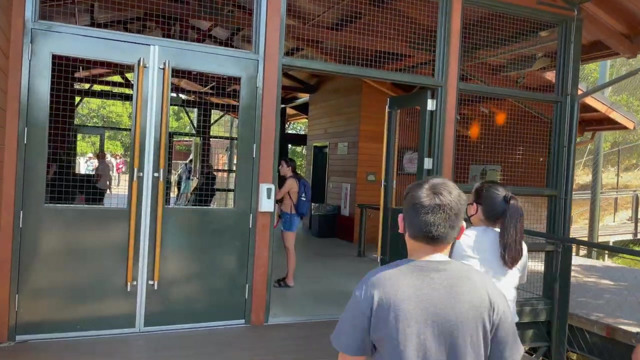 that's big. the things are vicious. that's big, that's big. oh my god, look at that machine. that's big, that's really big. I thought vultures were small animals. I thought vultures were small animals. that's so big, that's really big. 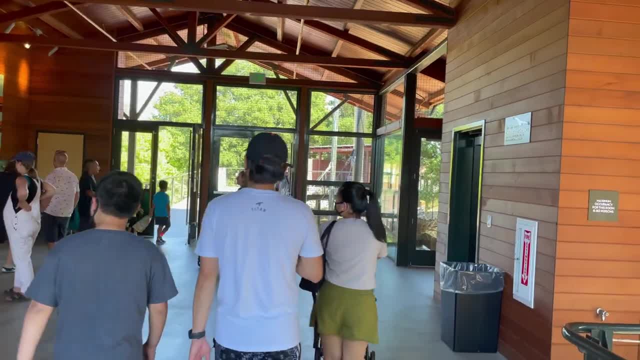 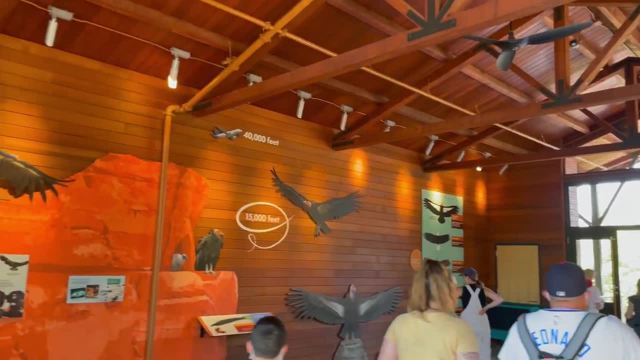 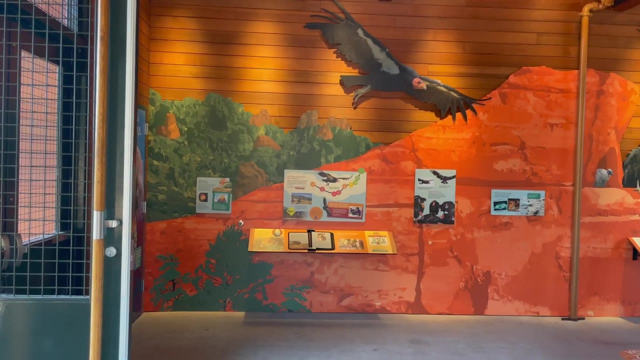 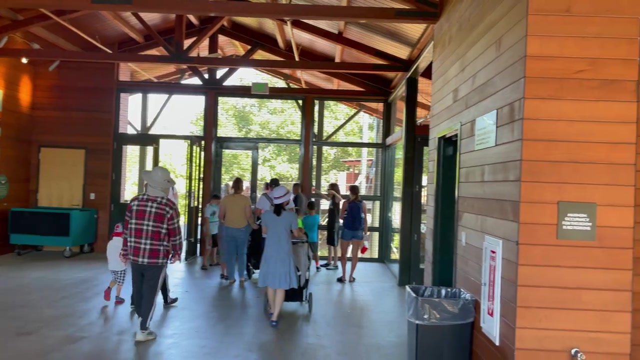 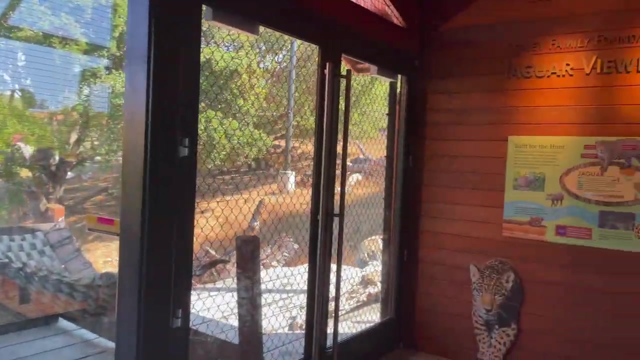 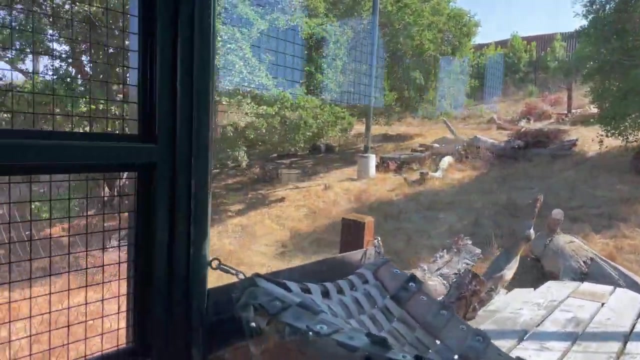 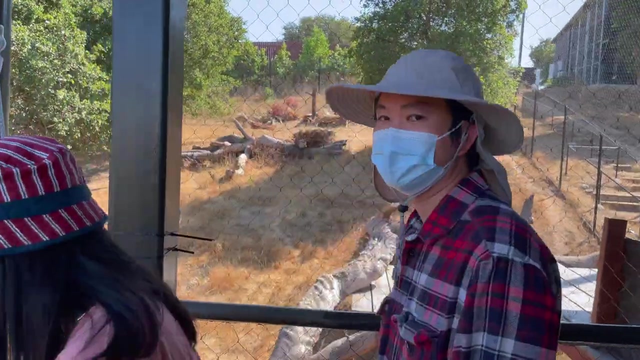 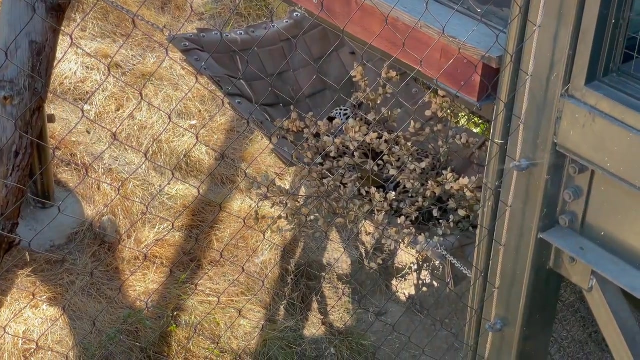 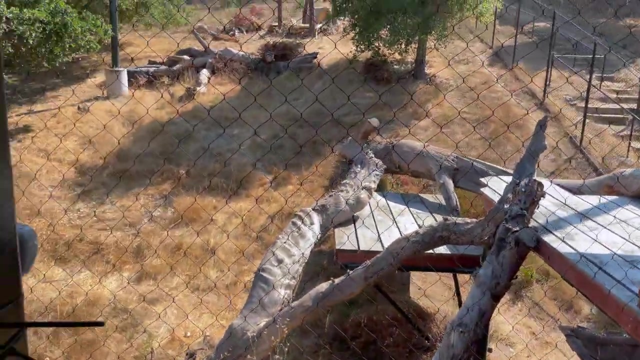 I think its huge. everybody is talking: how tall are you all? I'm very excited. uhhhh, come on, There's one over here I can't see. Get around. Oh, it's inside this thing. Yeah, It's sleeping in the hammock. 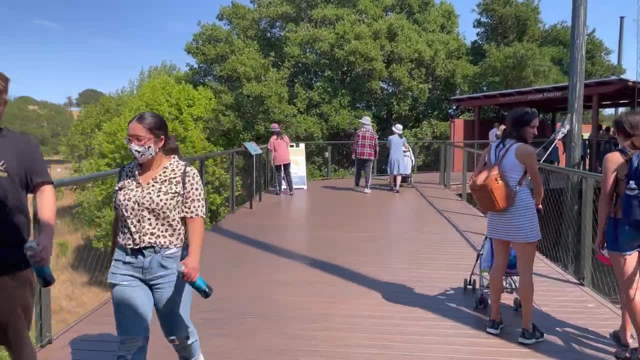 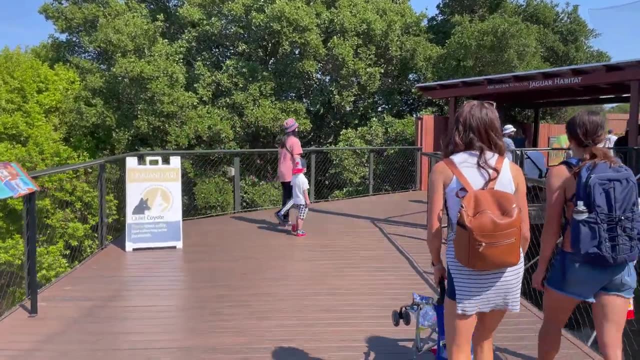 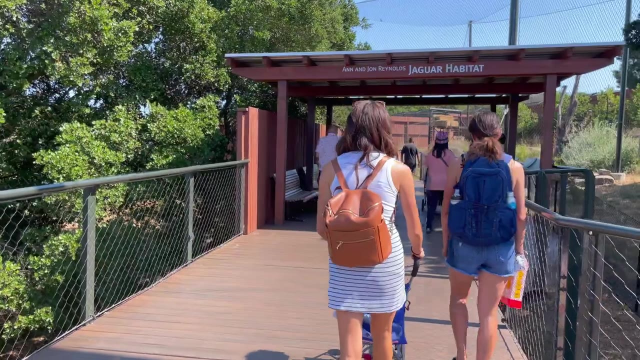 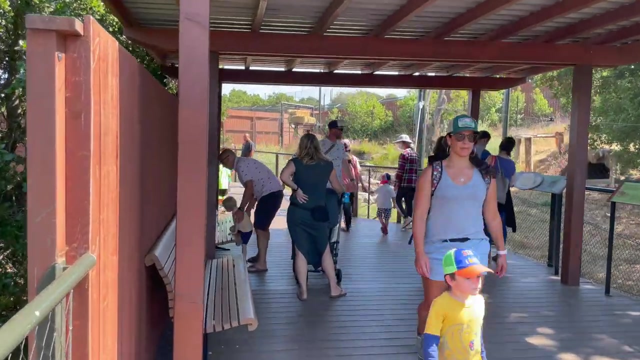 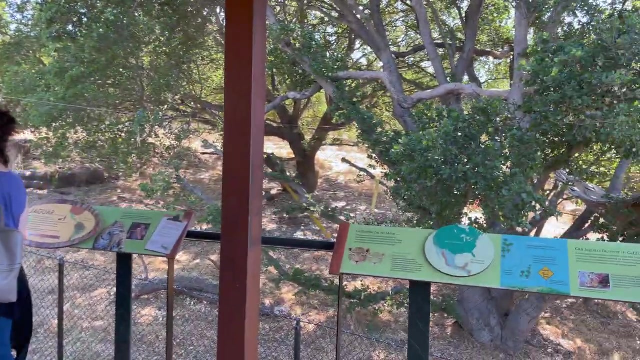 Yeah, You want to come in. It's hard to sleep in there too, Because it keeps like you stacked in this. you know, Yeah, On your hip or whatever Either side, or even like on your arm or something. 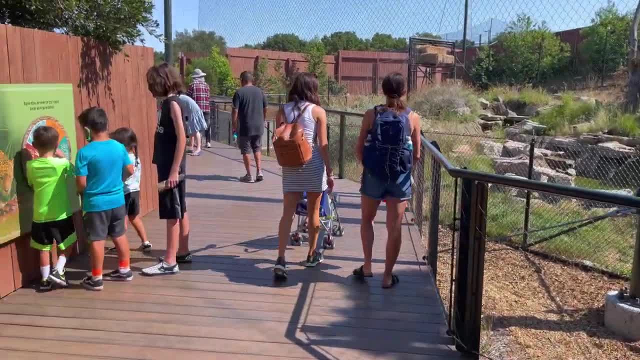 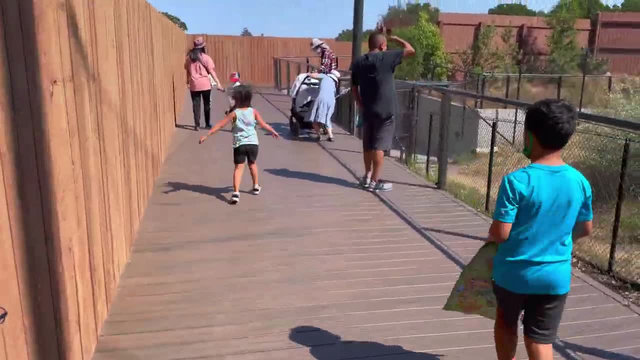 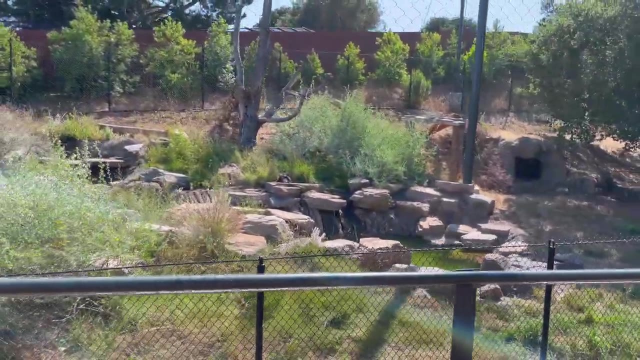 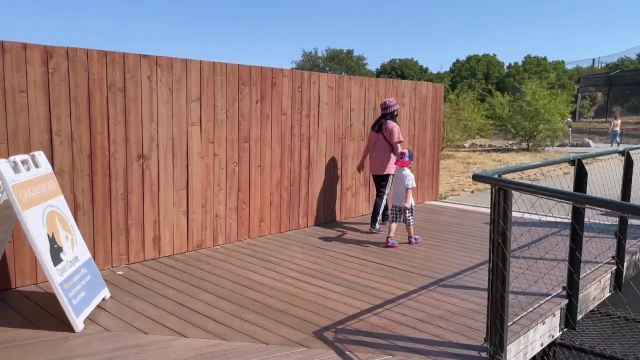 And then they go through the grave Success: Praise Snowy, Praise Snowy Coming for a spinner. Come on, Look at that birdie all the way at the top. Cool, It's a baby that looks like that. 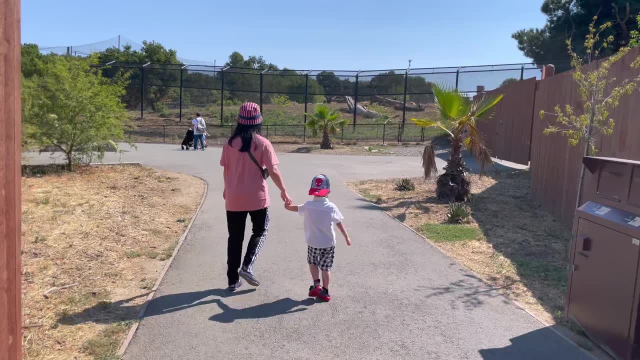 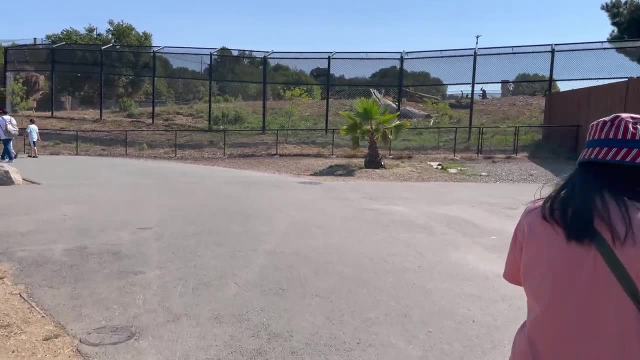 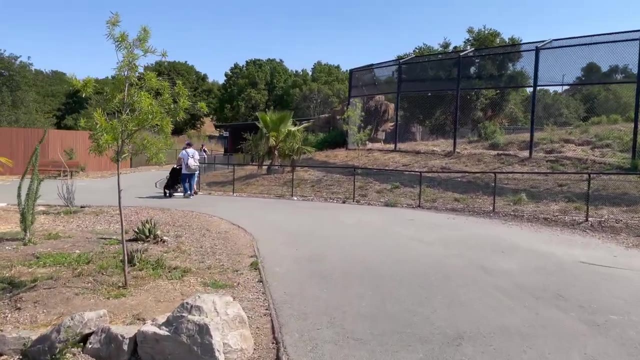 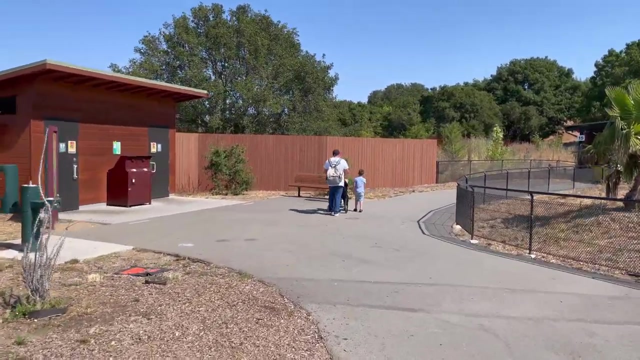 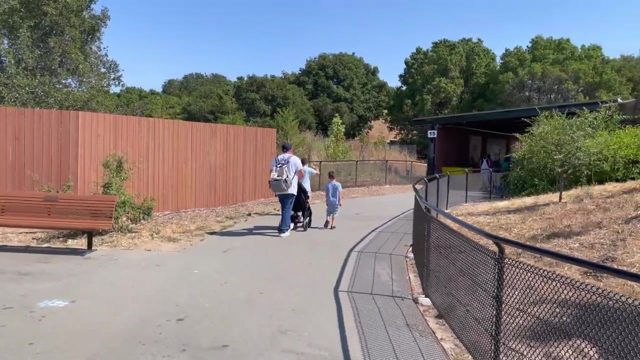 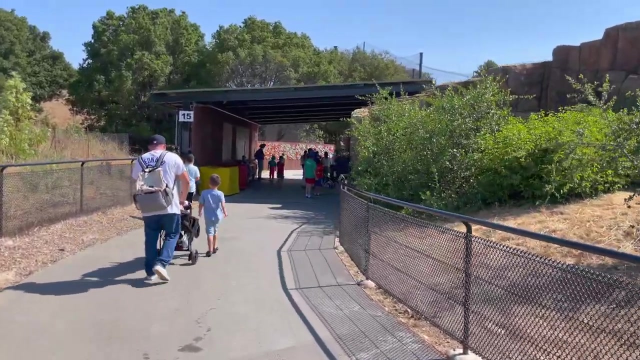 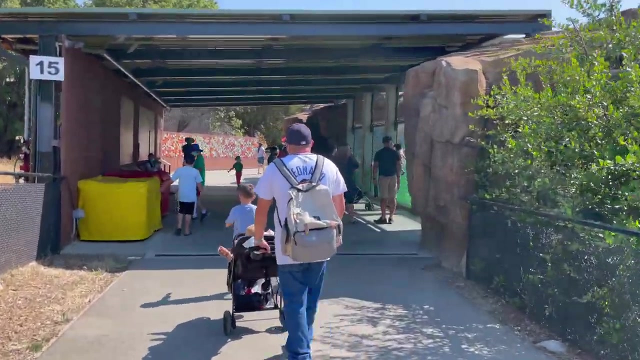 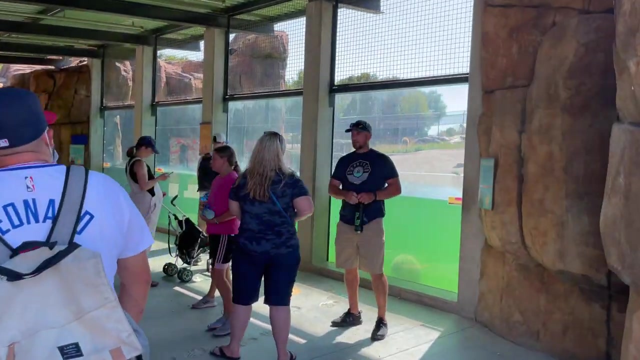 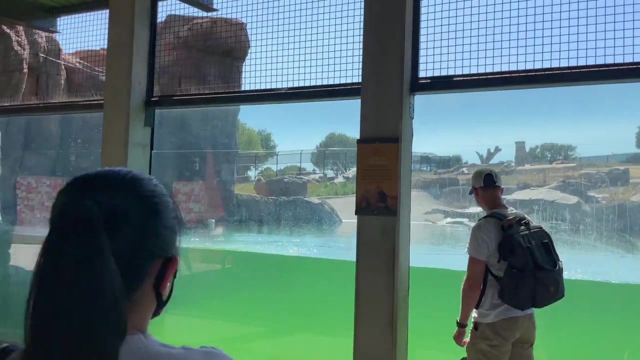 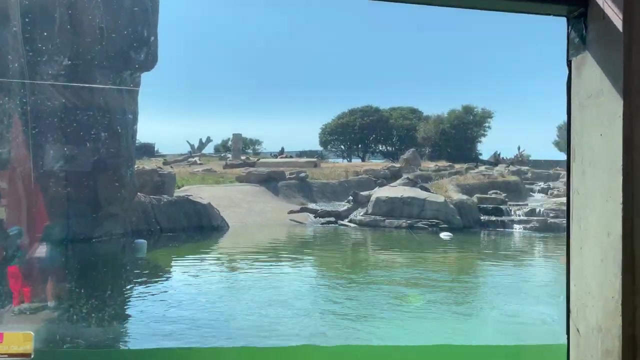 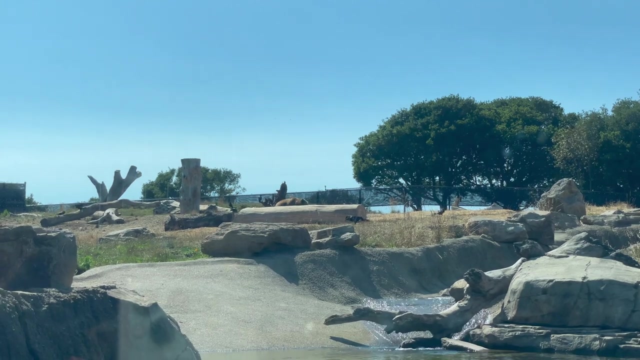 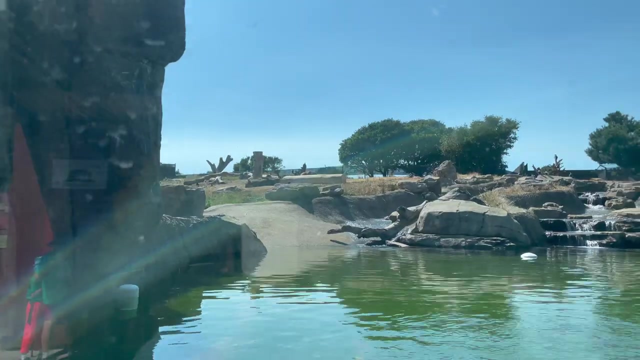 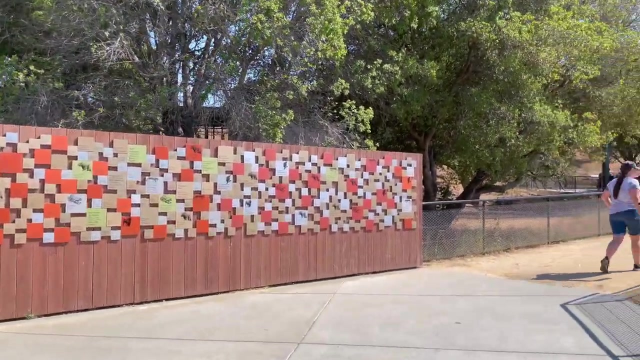 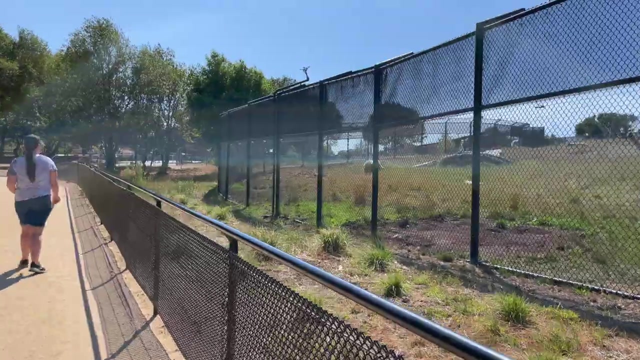 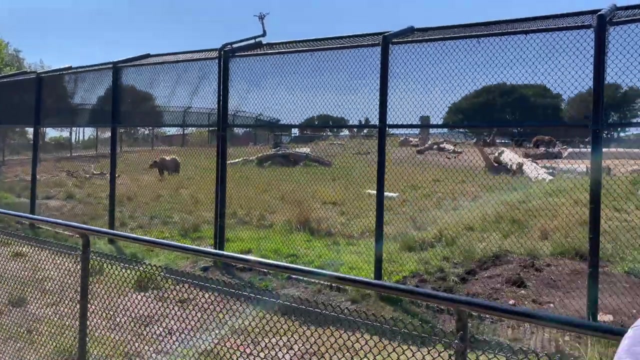 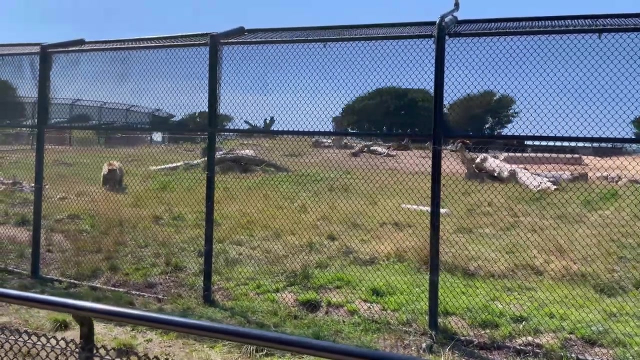 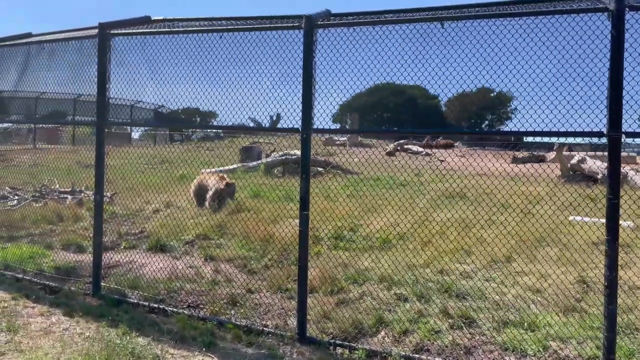 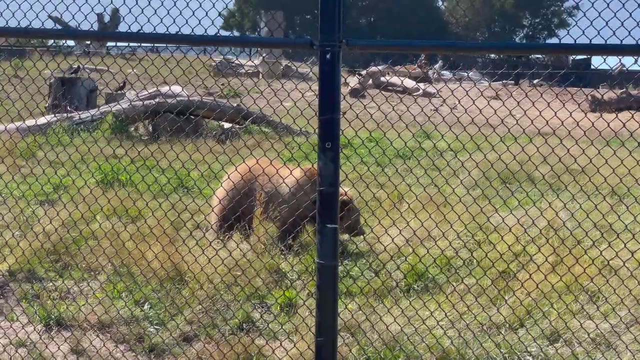 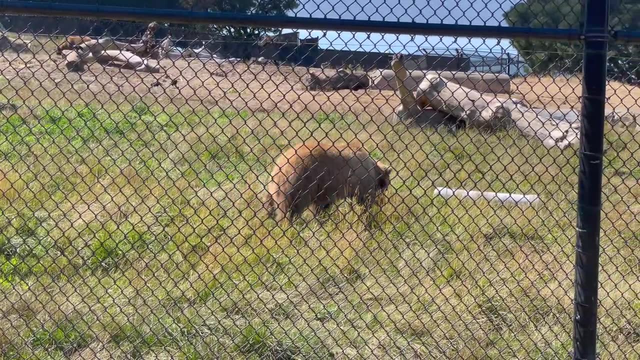 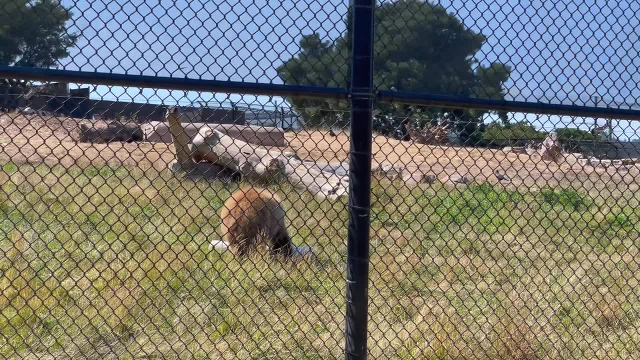 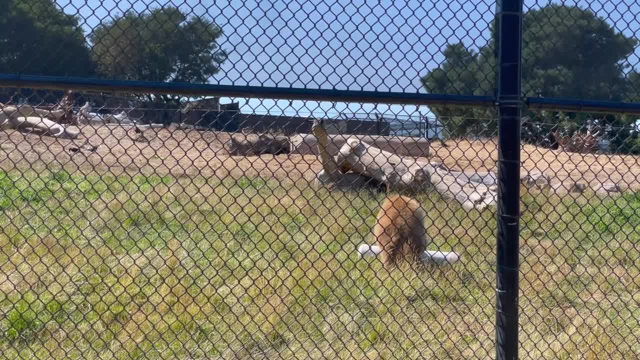 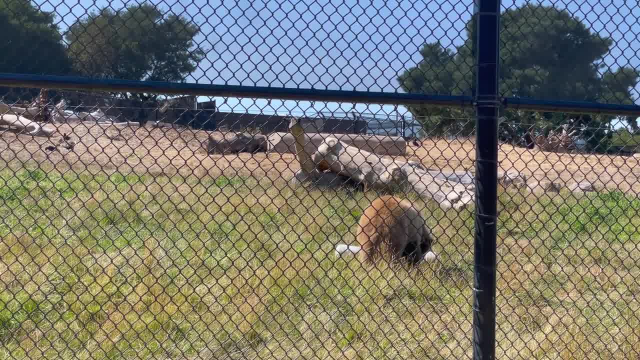 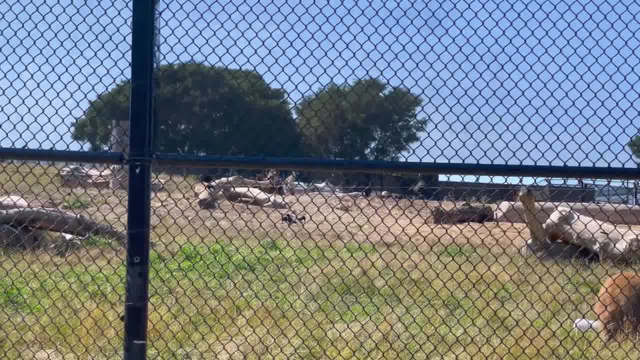 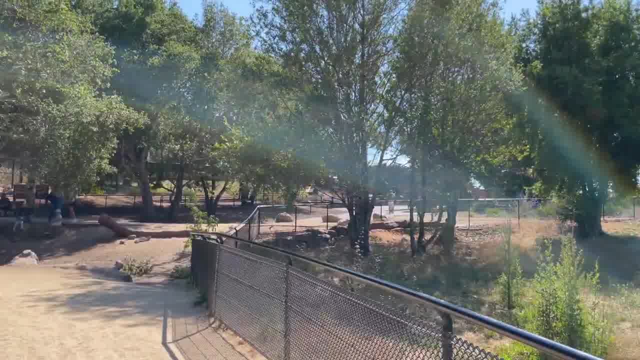 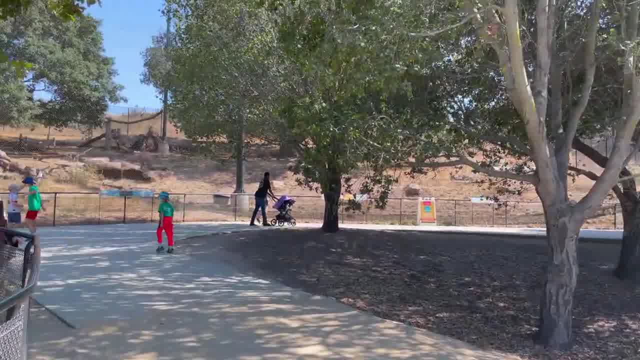 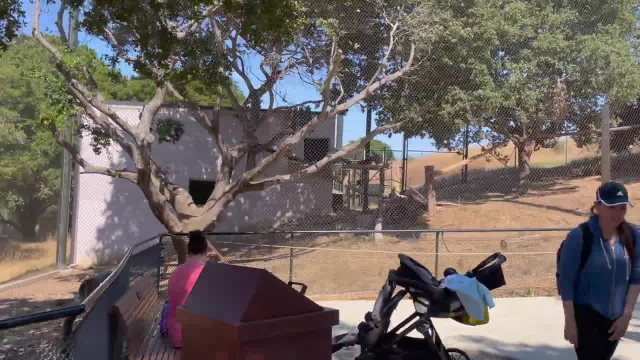 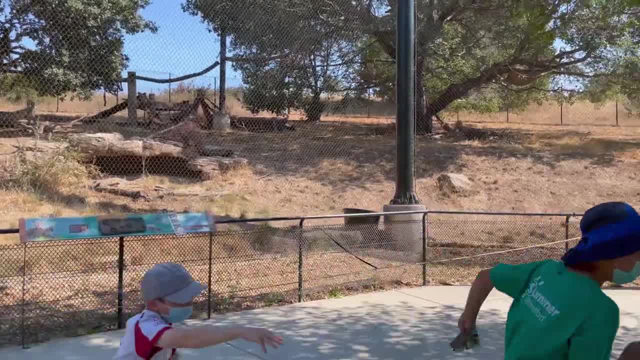 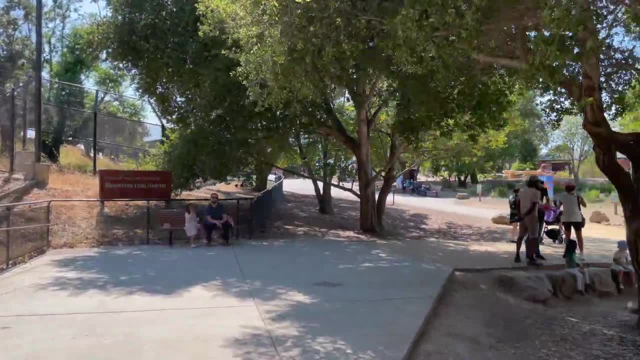 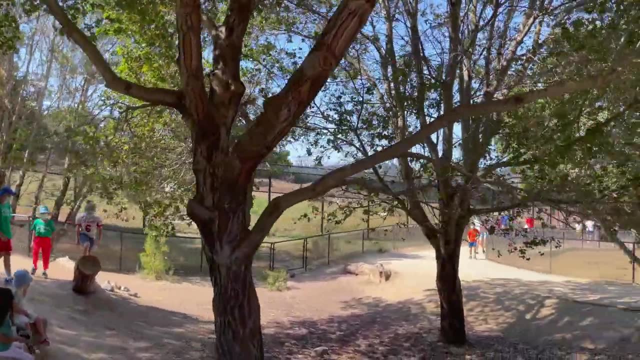 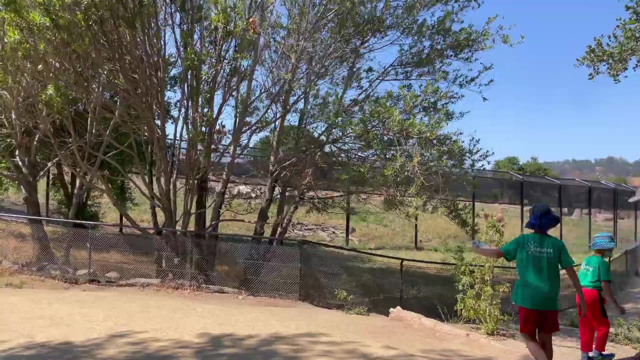 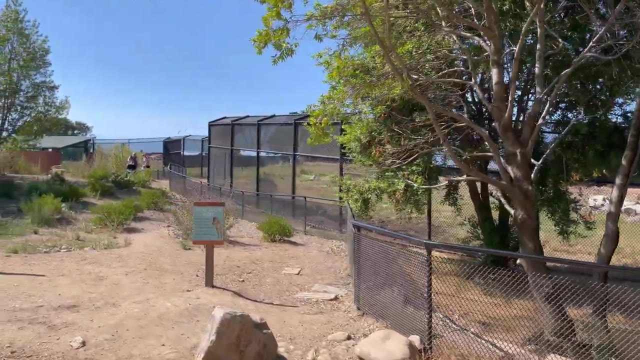 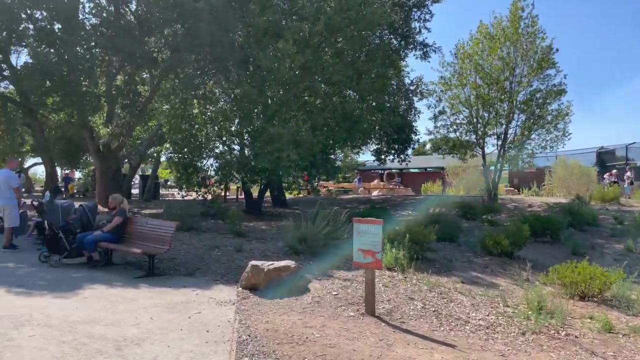 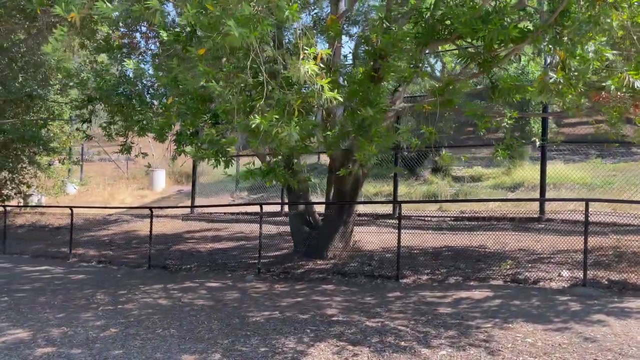 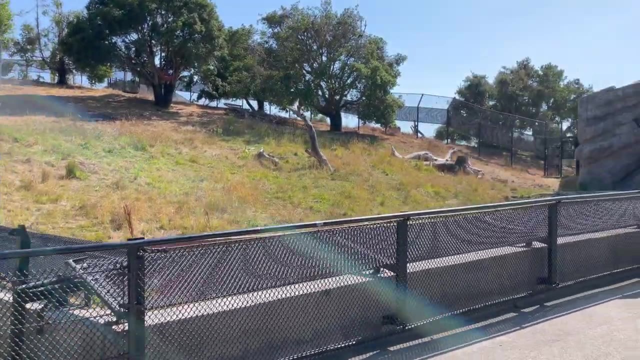 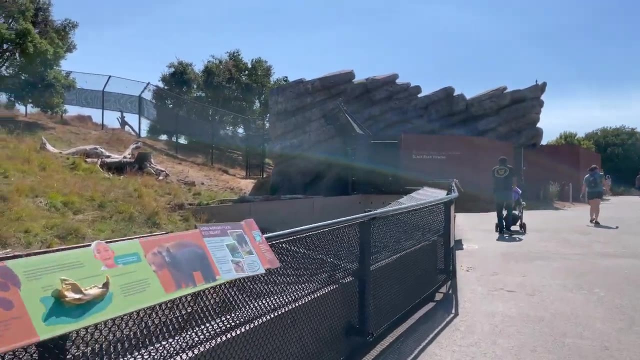 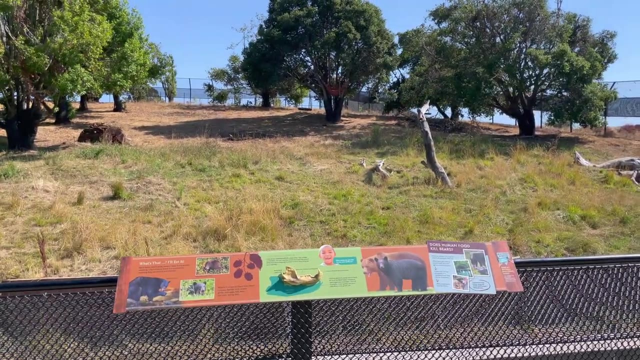 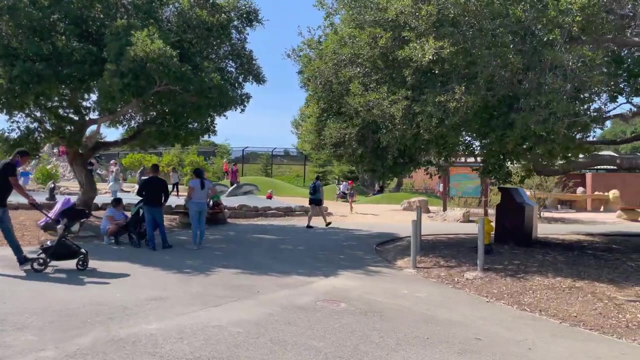 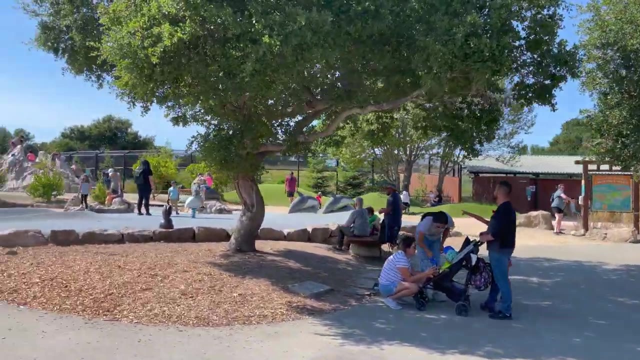 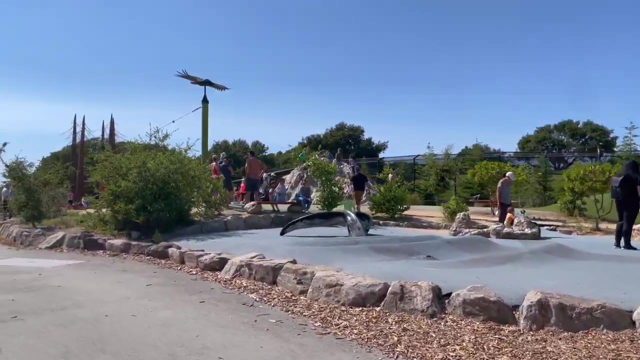 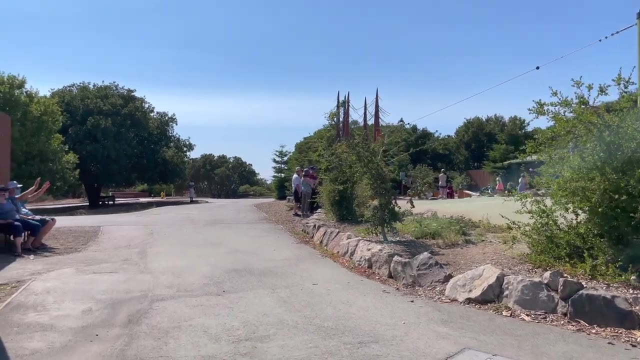 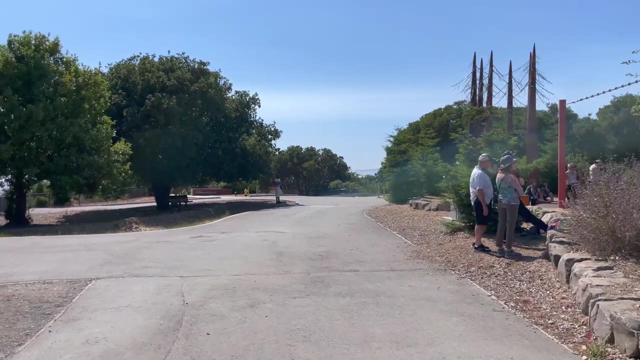 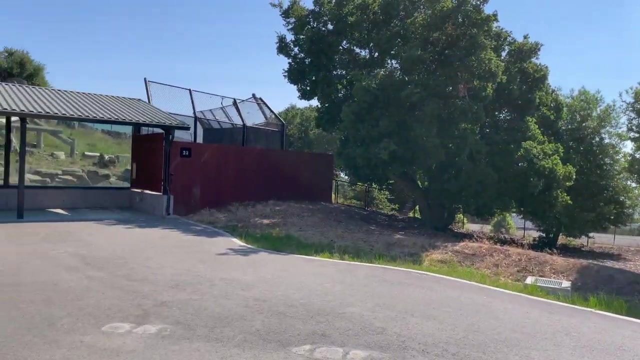 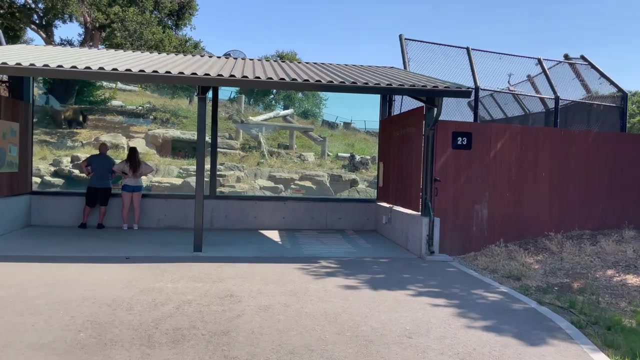 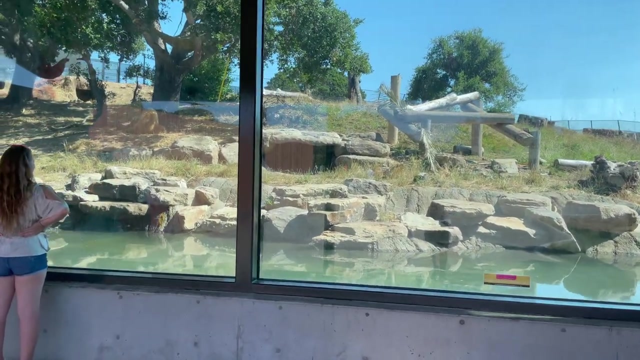 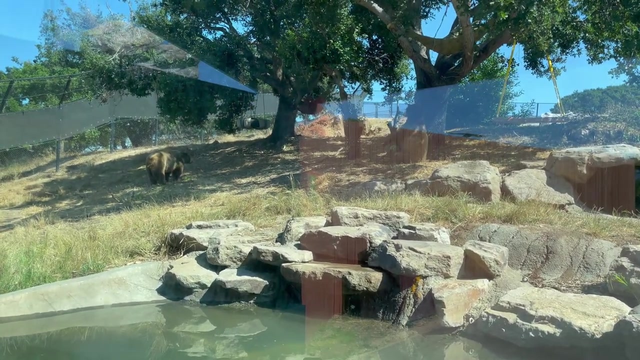 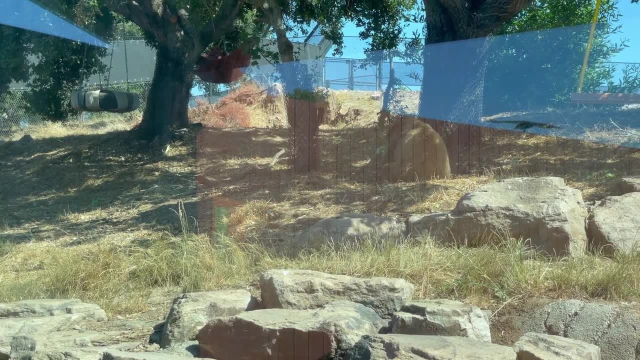 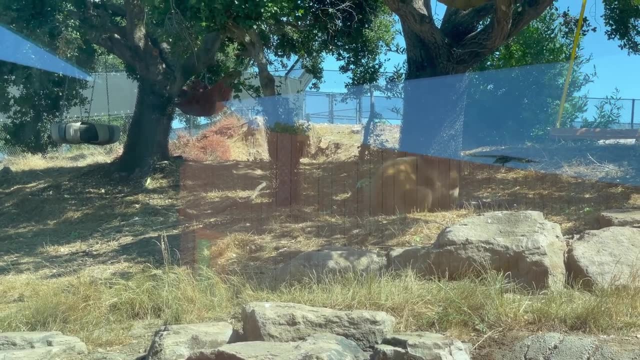 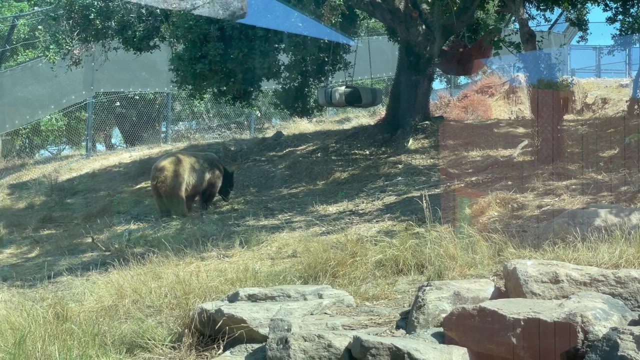 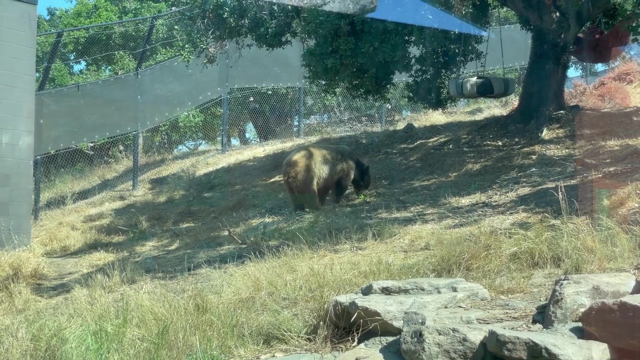 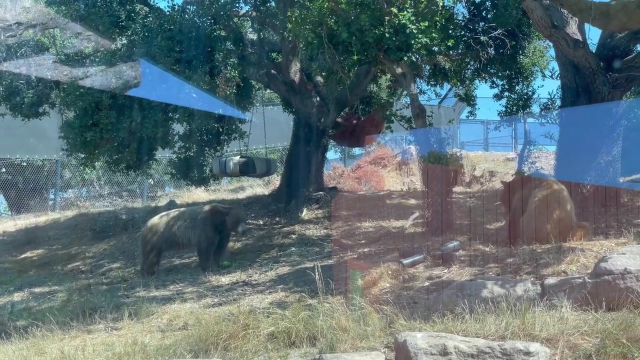 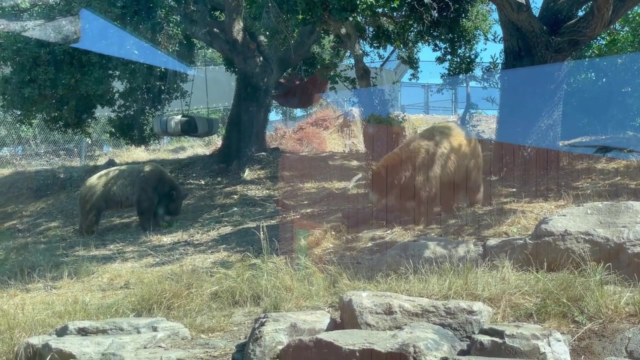 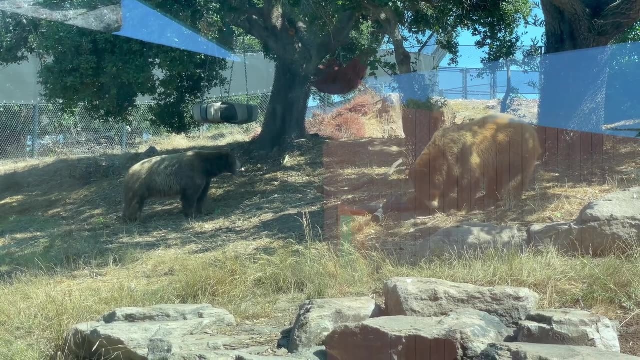 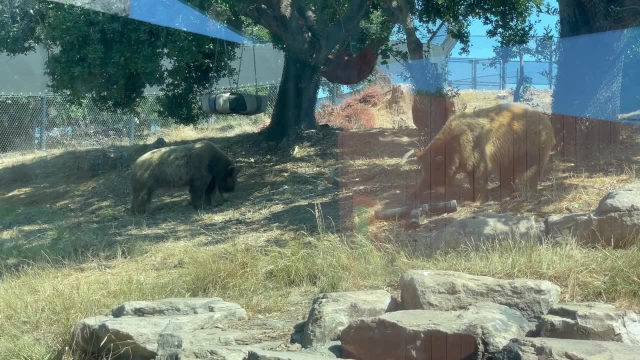 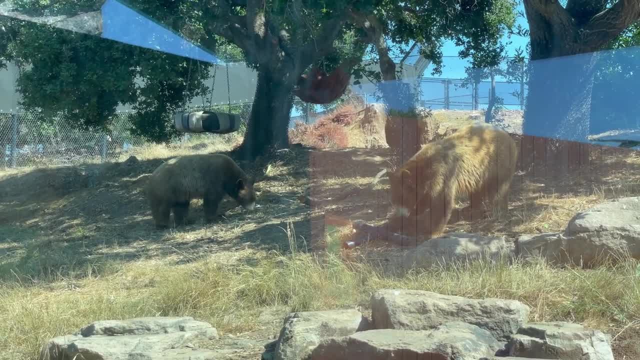 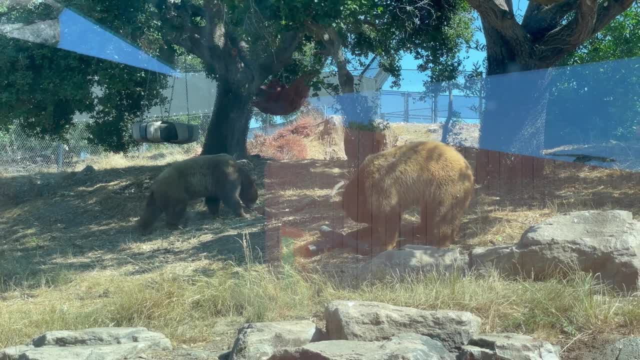 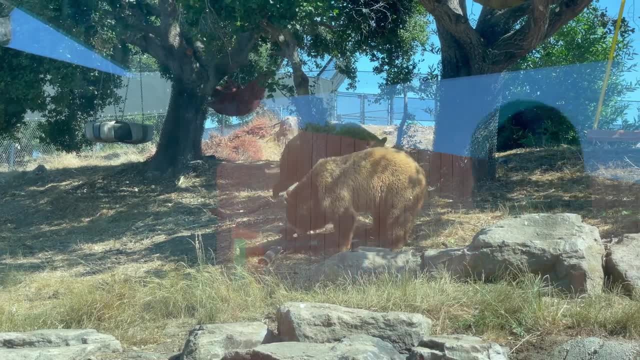 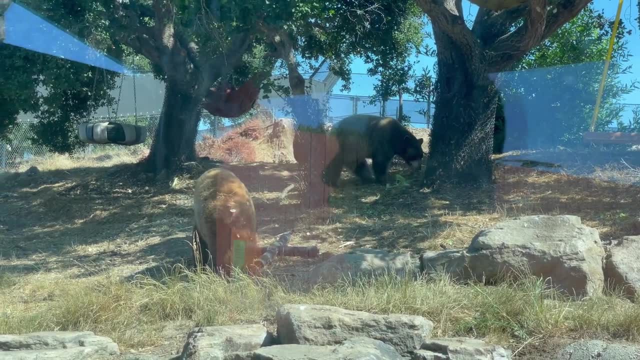 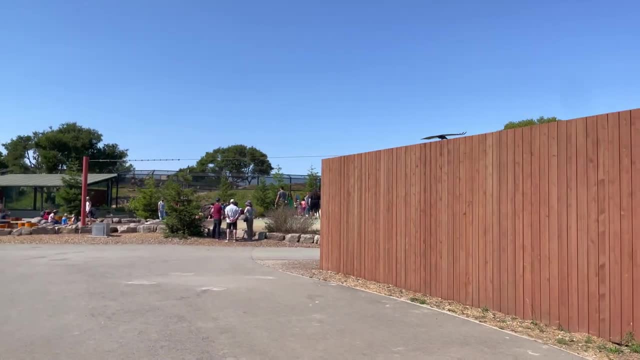 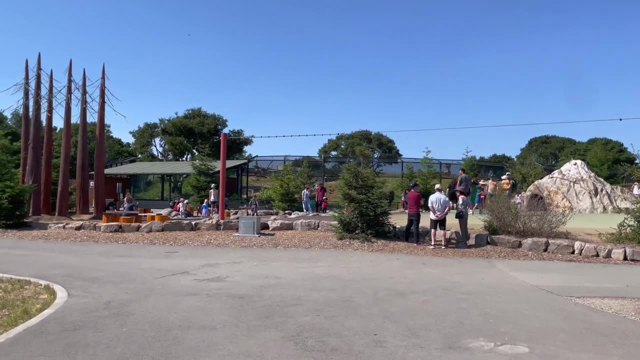 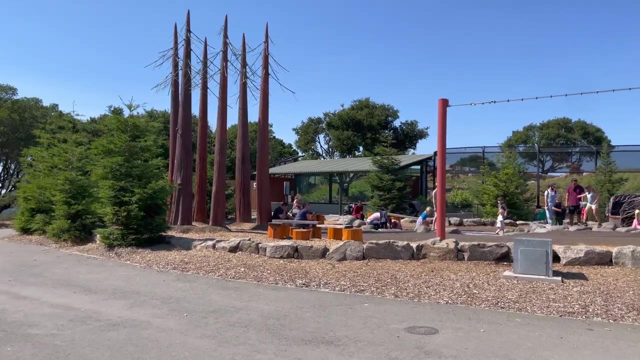 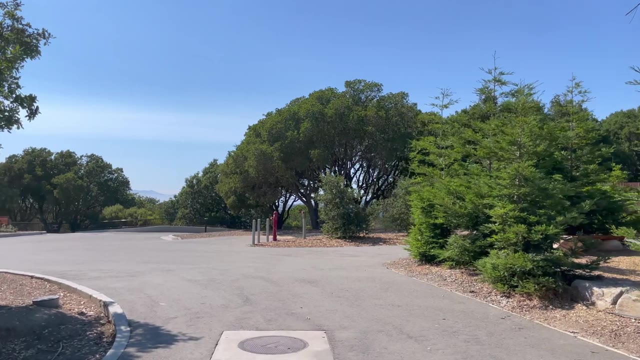 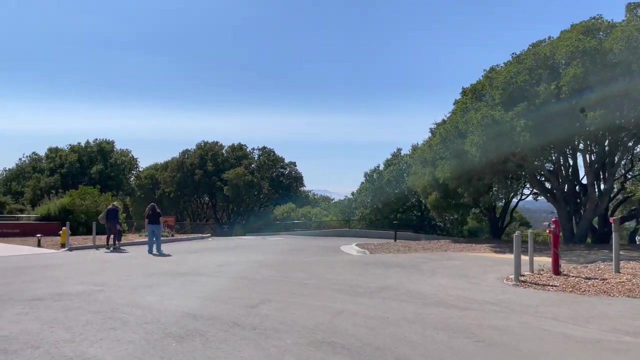 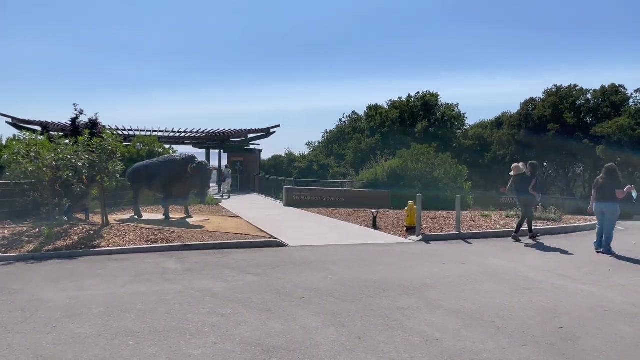 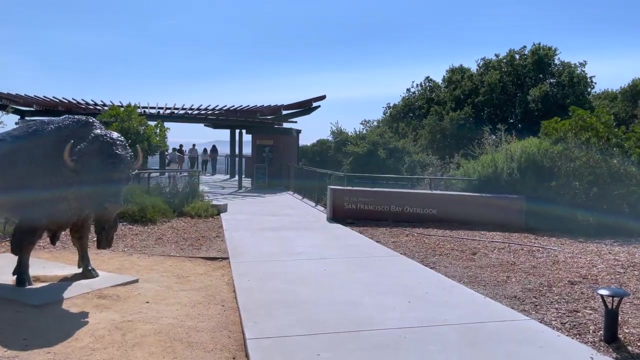 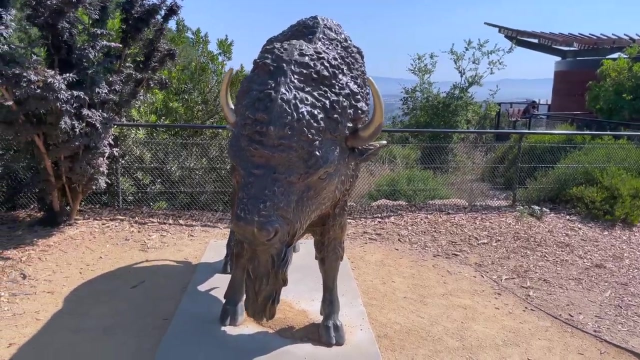 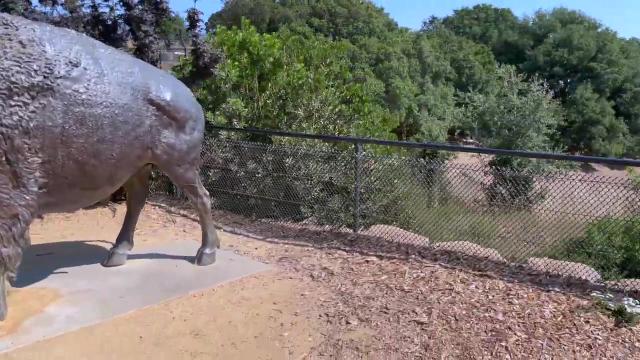 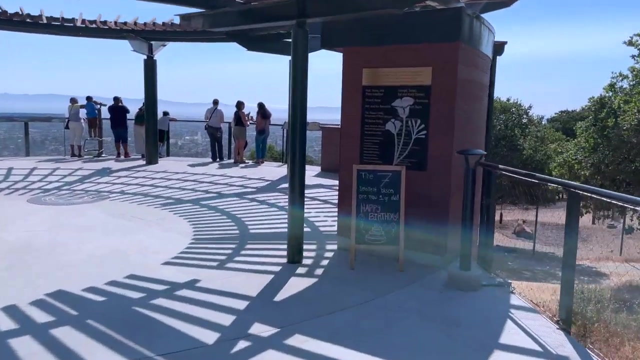 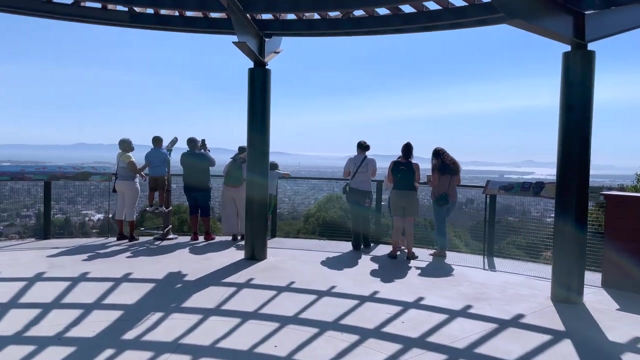 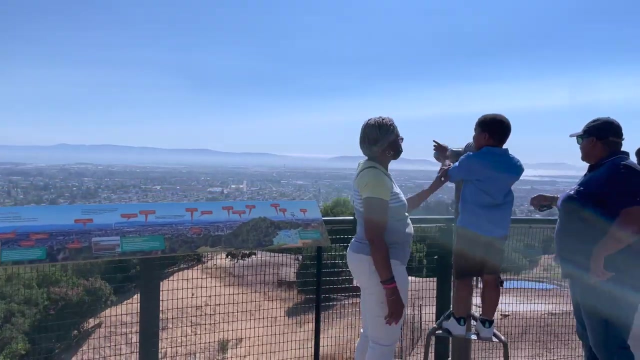 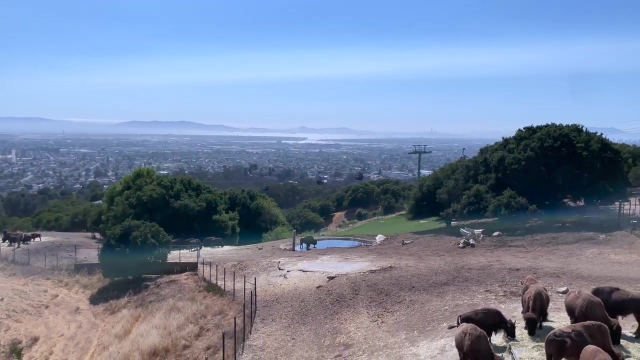 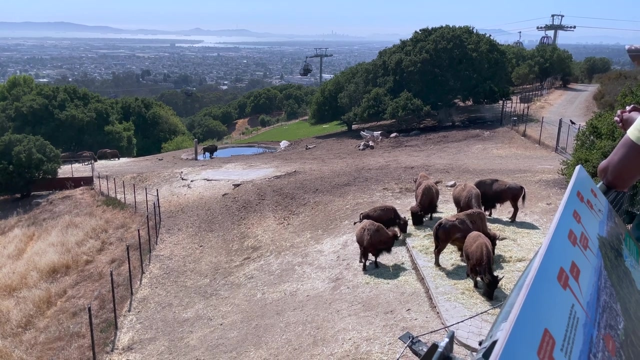 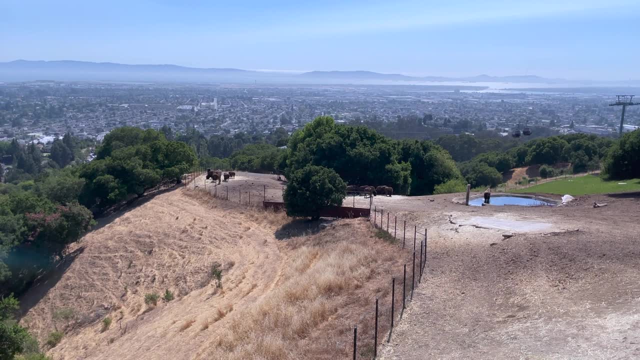 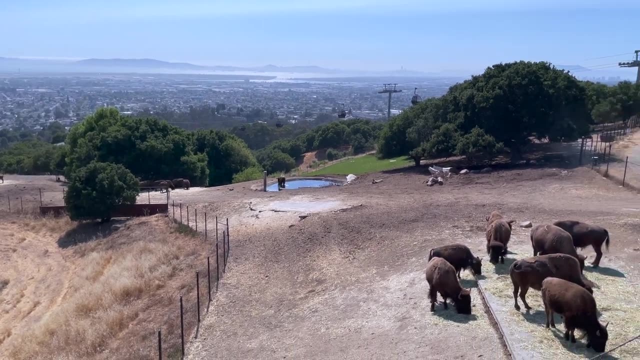 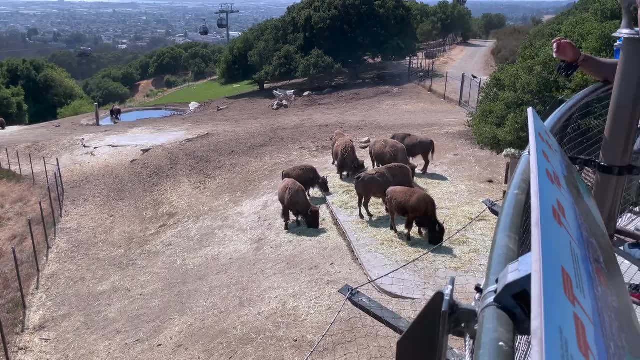 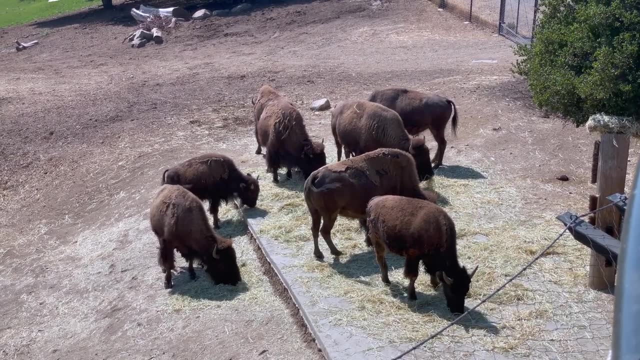 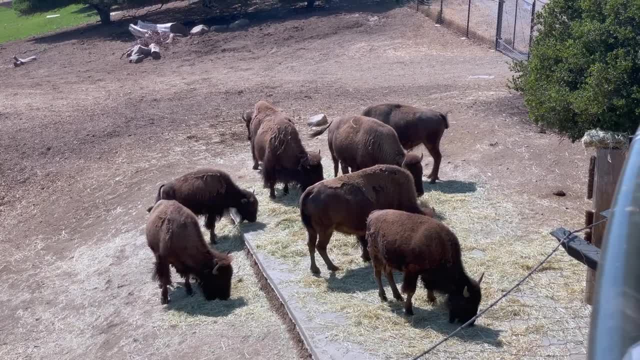 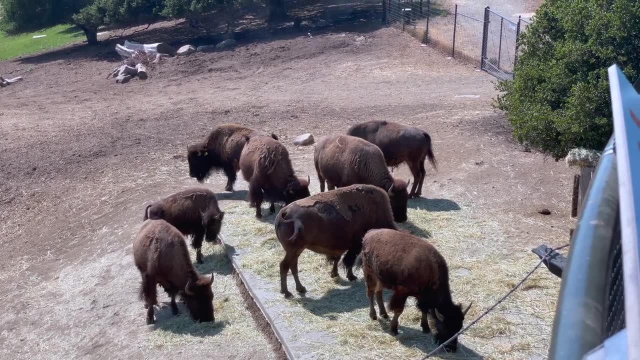 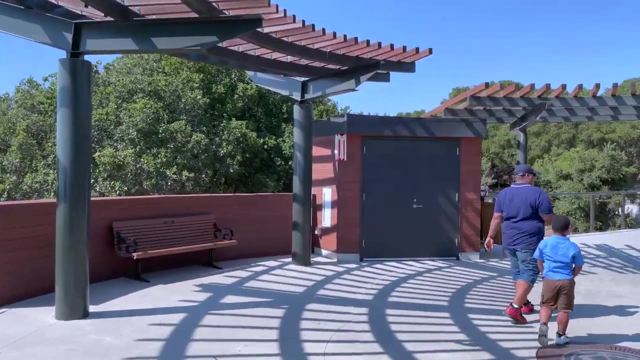 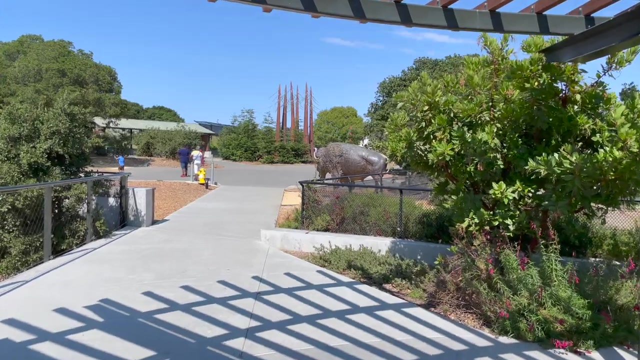 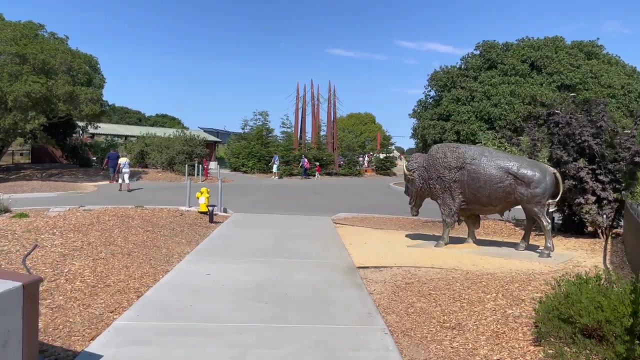 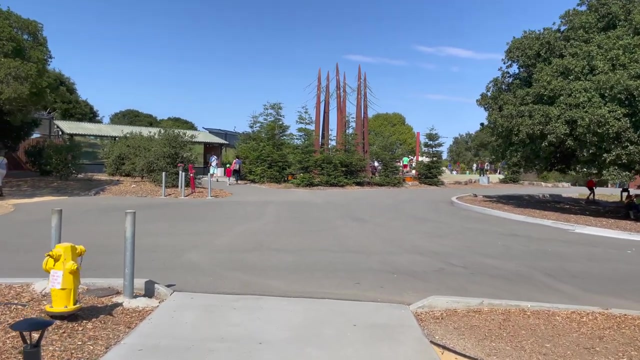 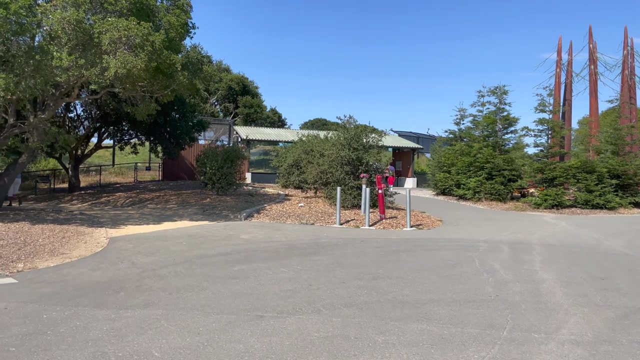 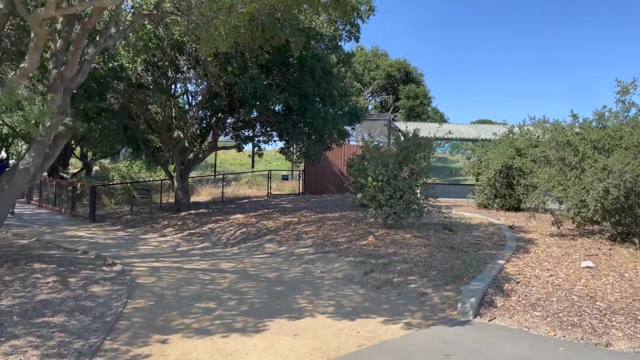 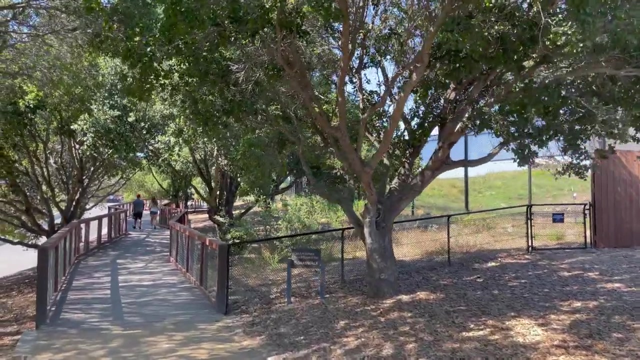 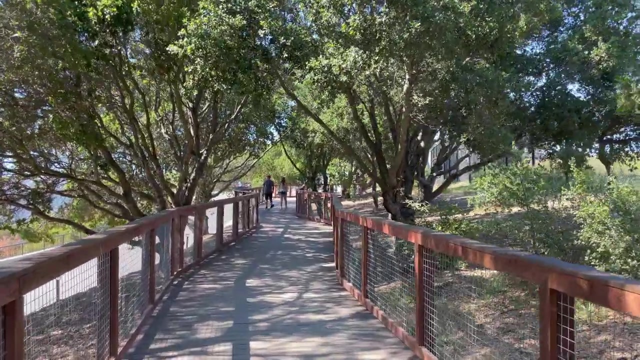 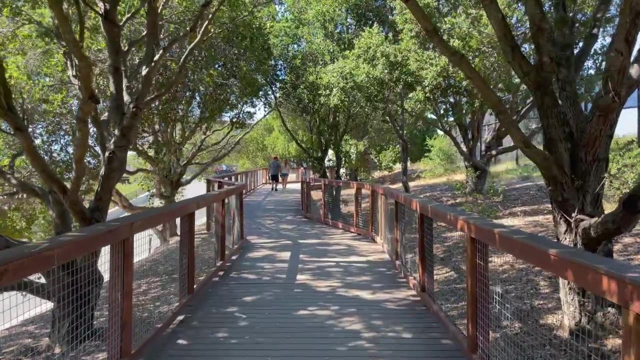 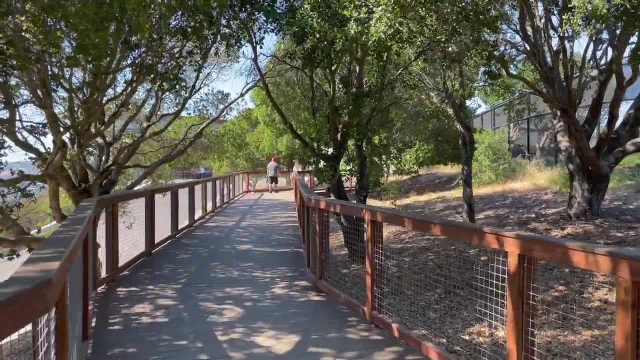 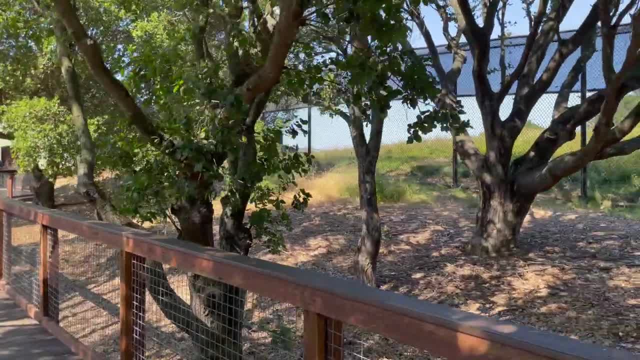 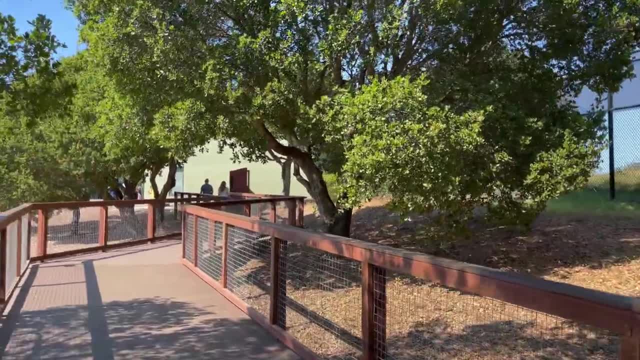 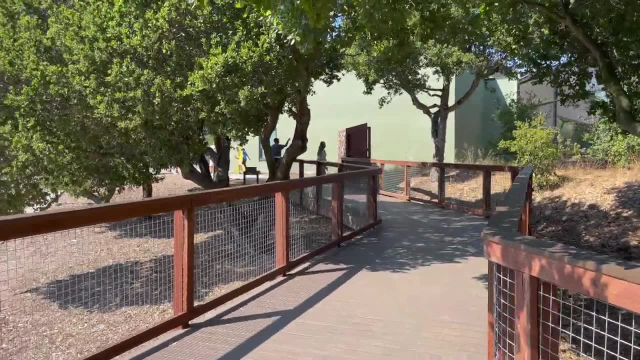 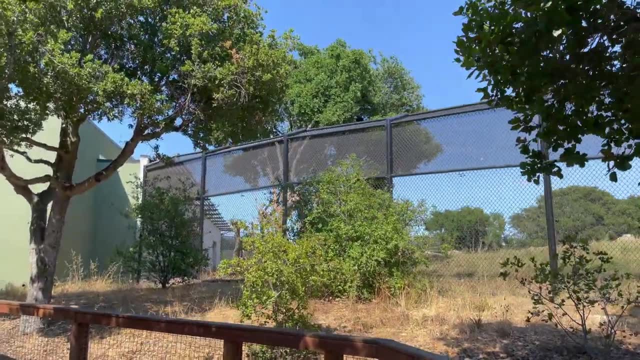 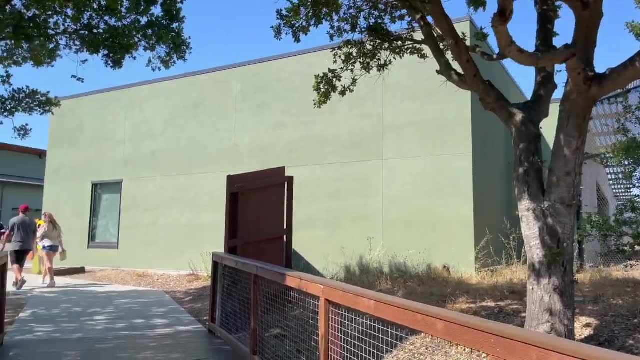 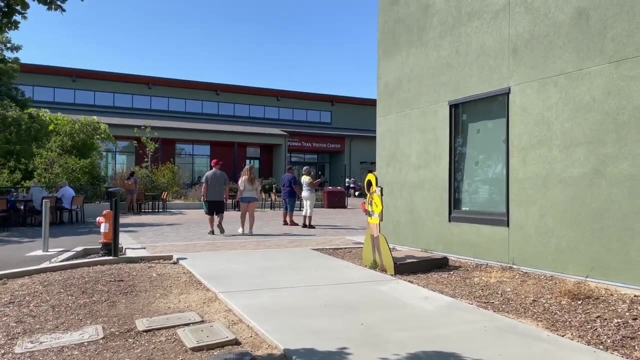 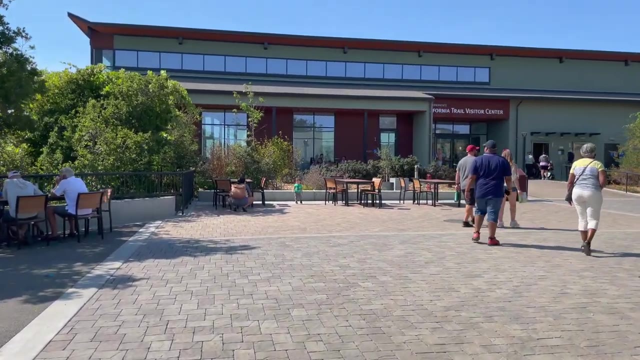 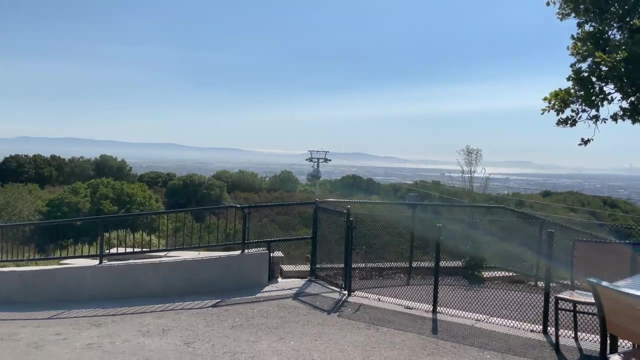 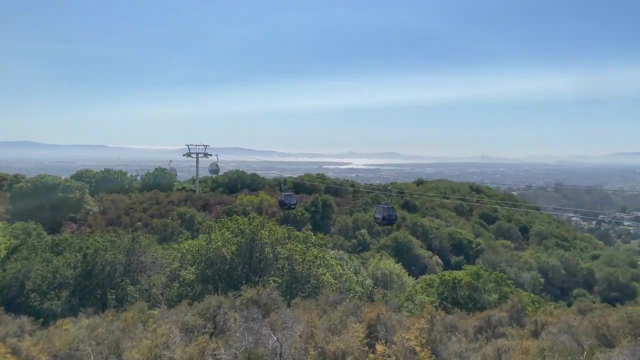 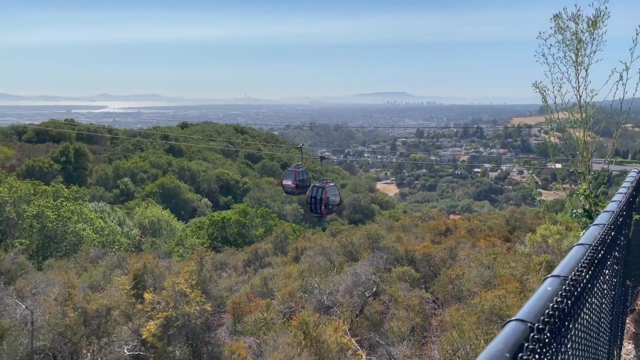 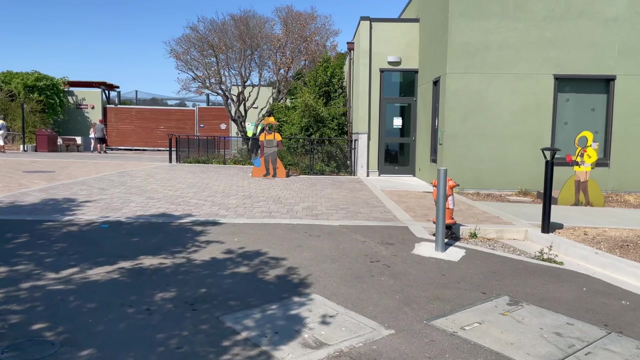 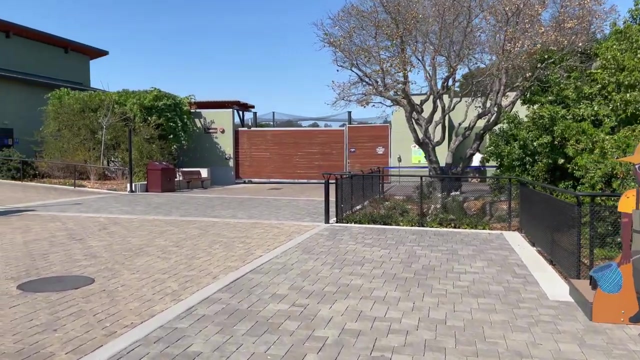 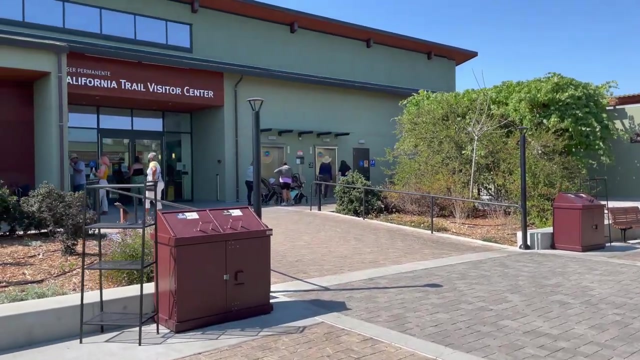 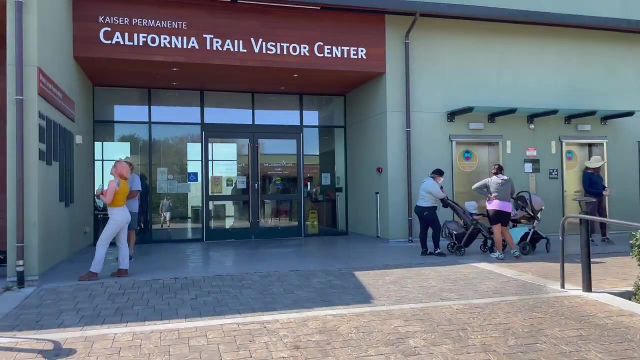 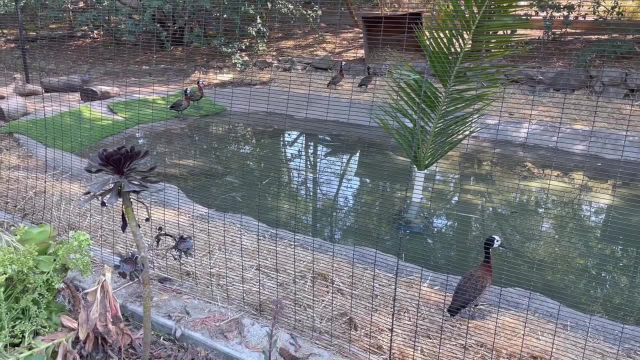 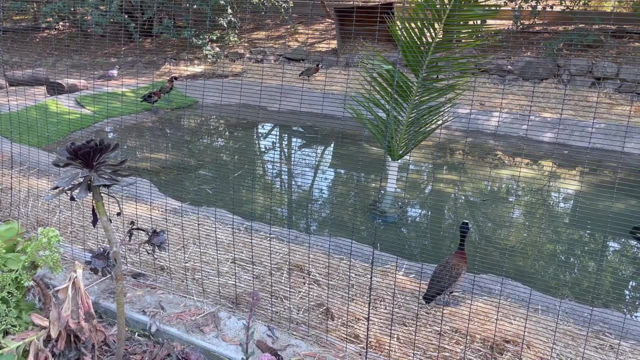 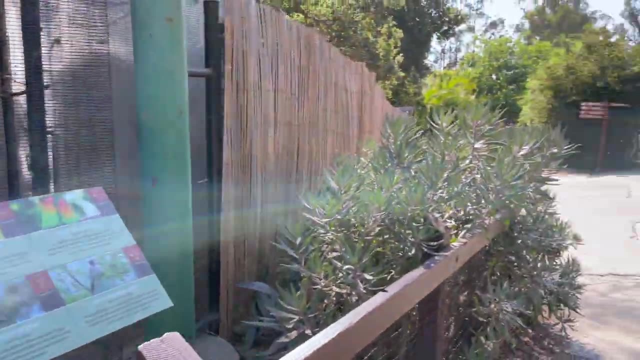 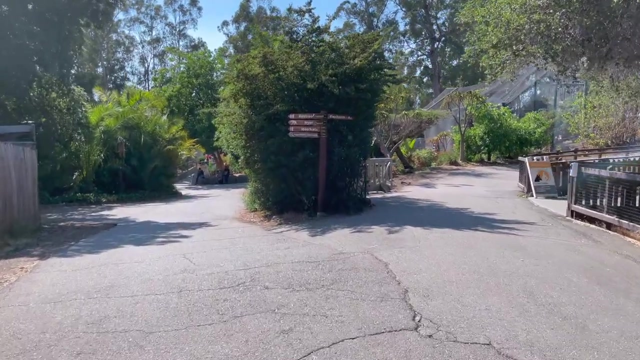 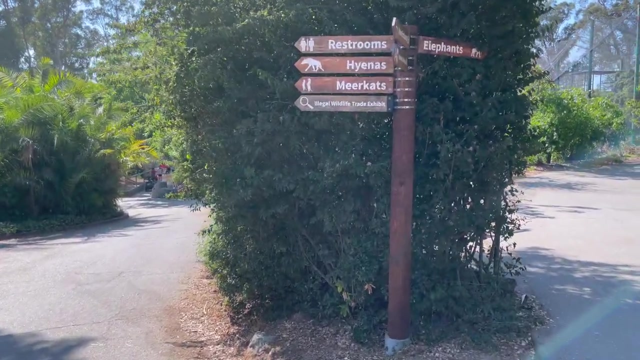 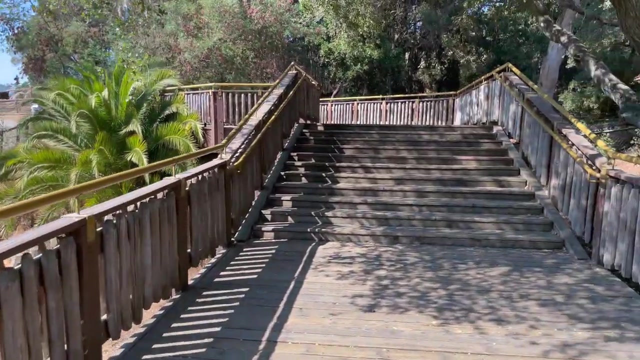 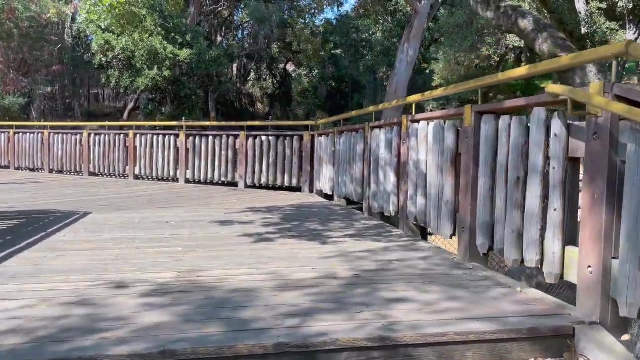 I see a hummingbird. I see a little bush. I see a little plant. I see a little bush up here. I see a little bird. I see a little bird. Hi guys, I see a little bird. Hi guys, Hi guys. 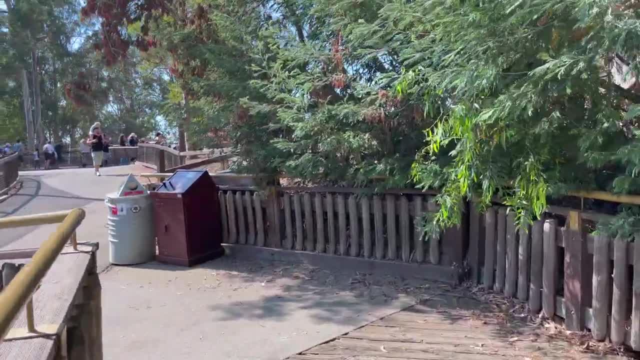 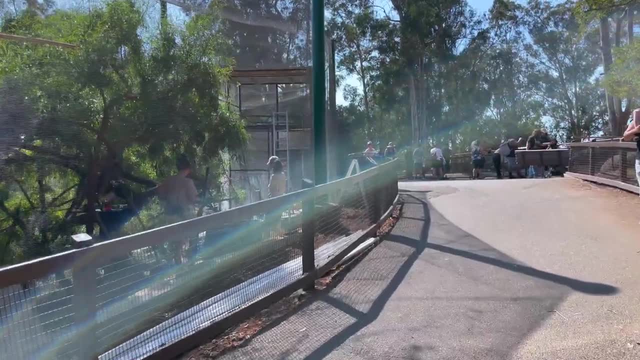 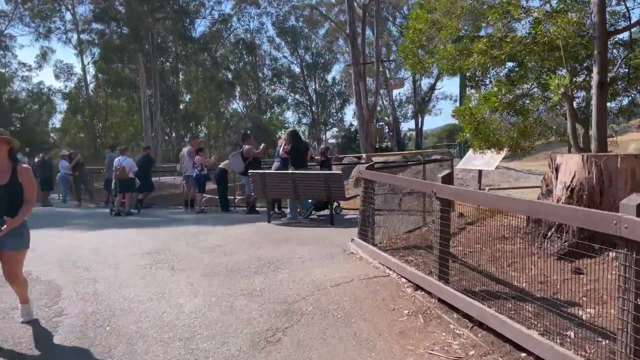 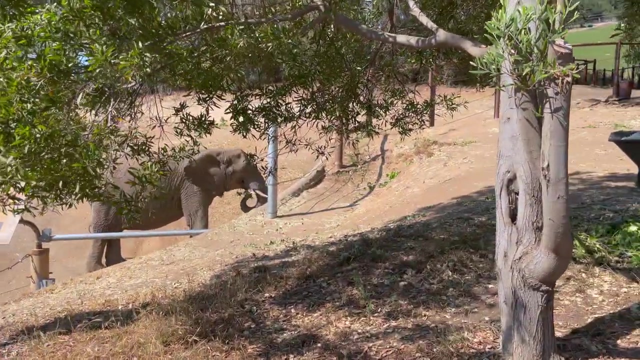 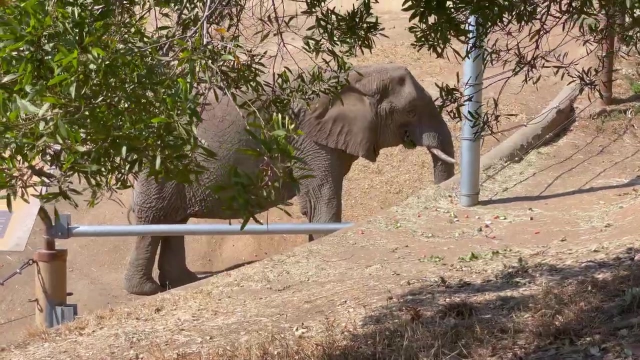 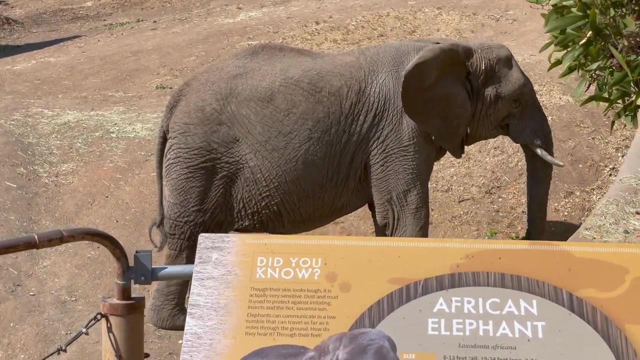 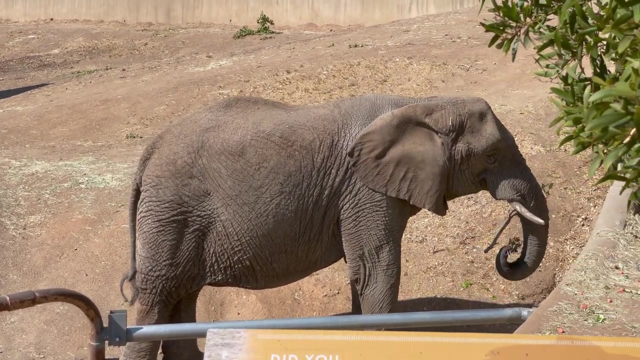 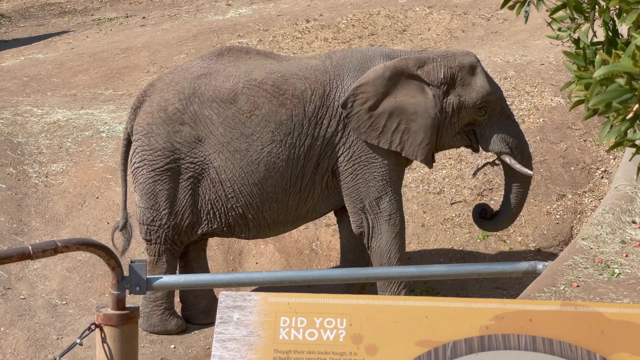 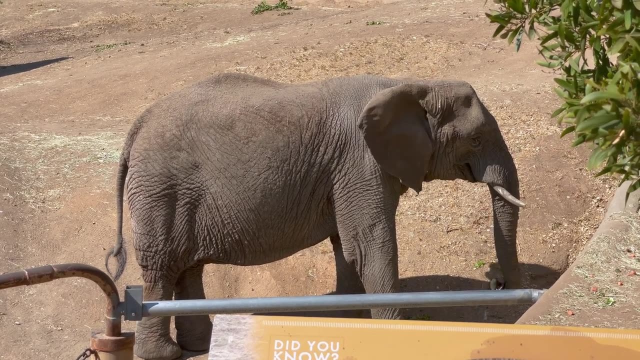 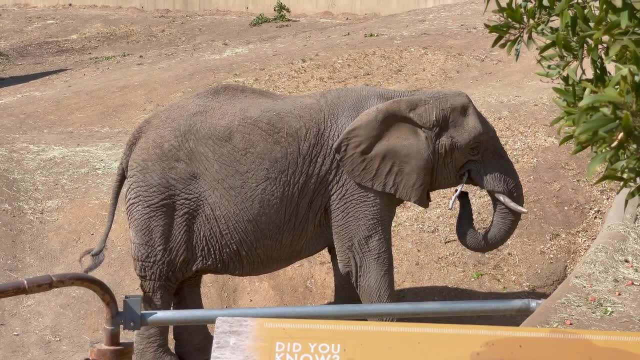 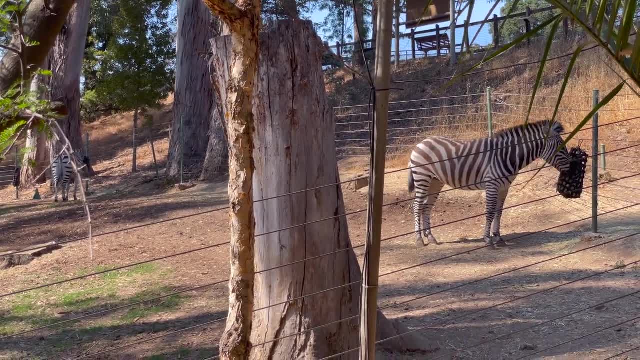 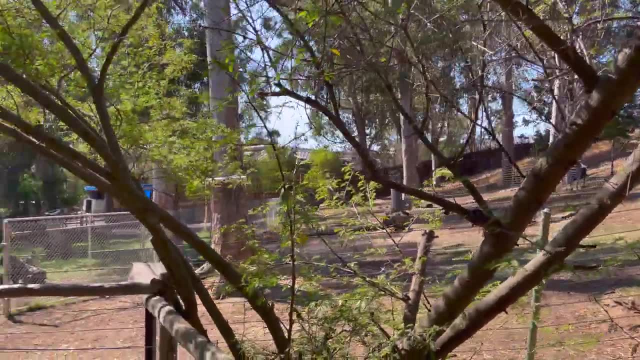 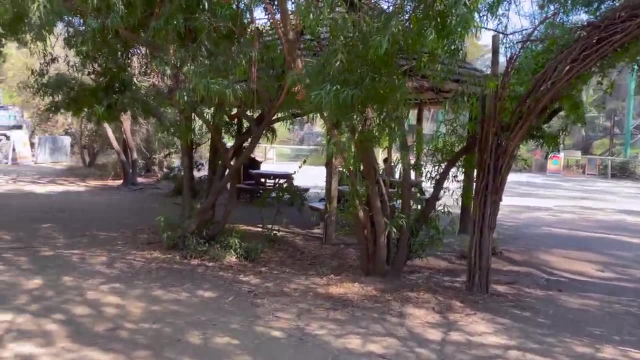 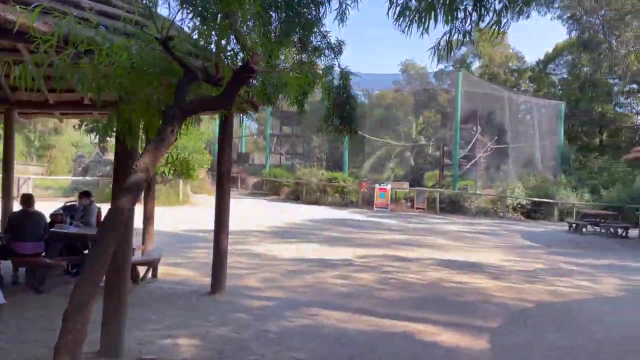 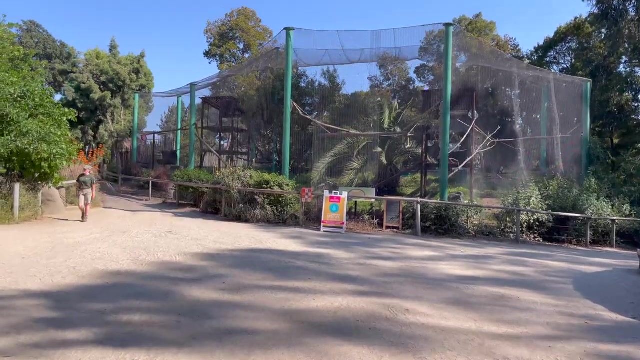 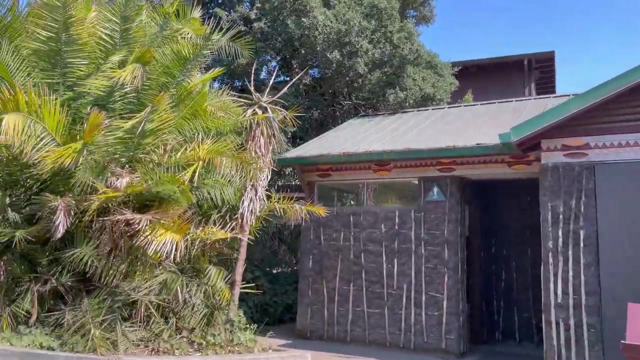 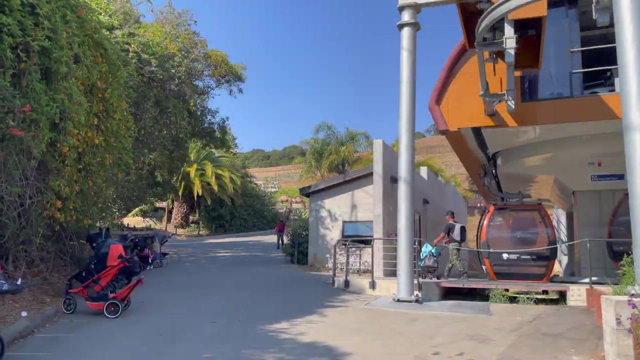 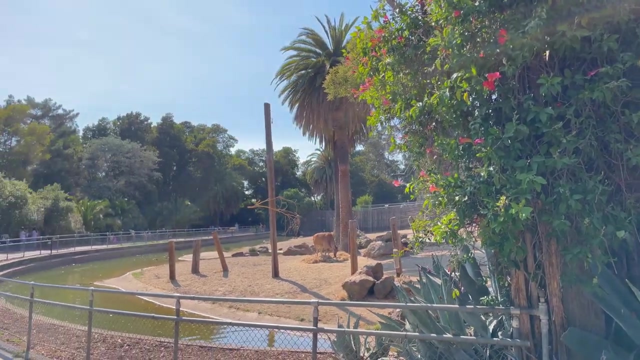 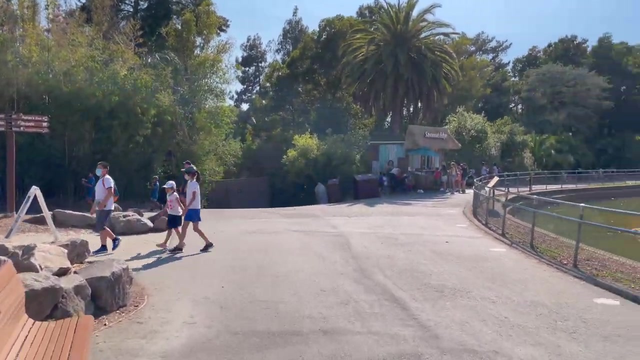 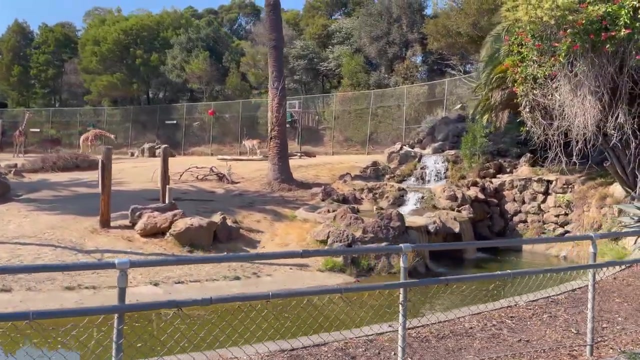 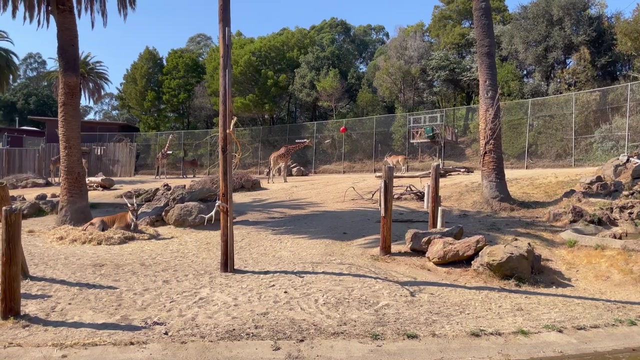 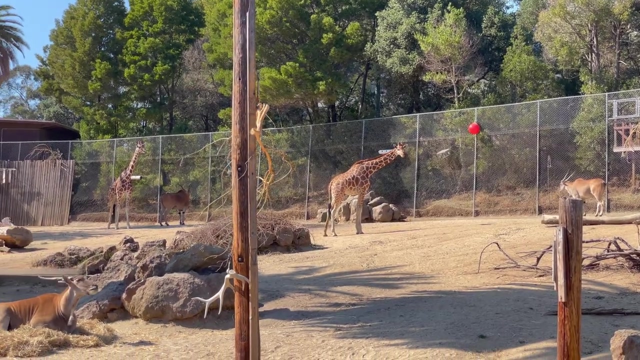 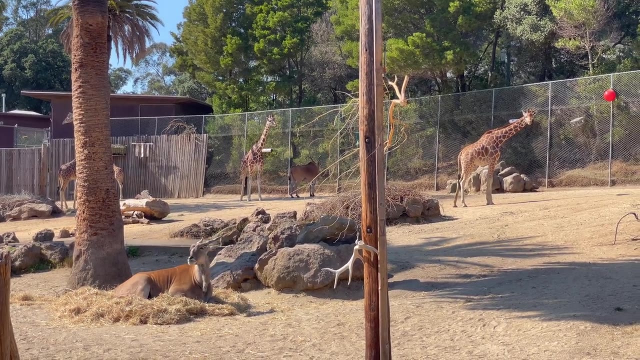 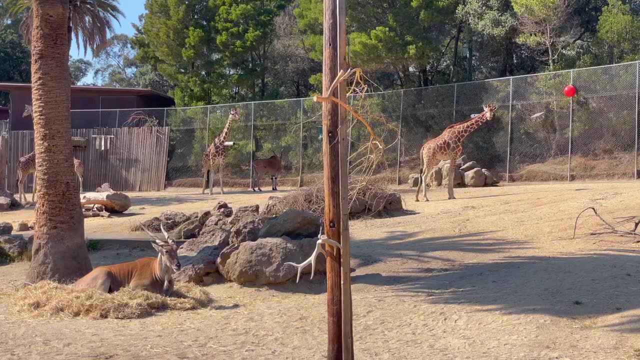 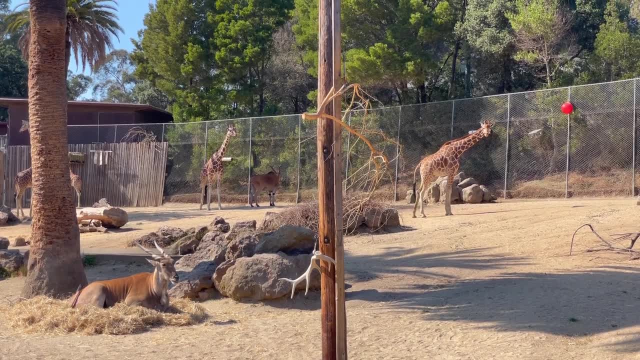 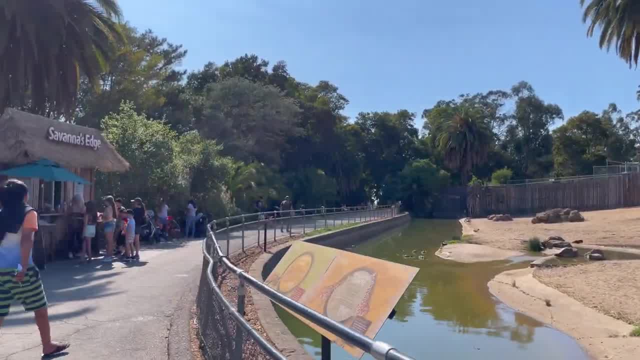 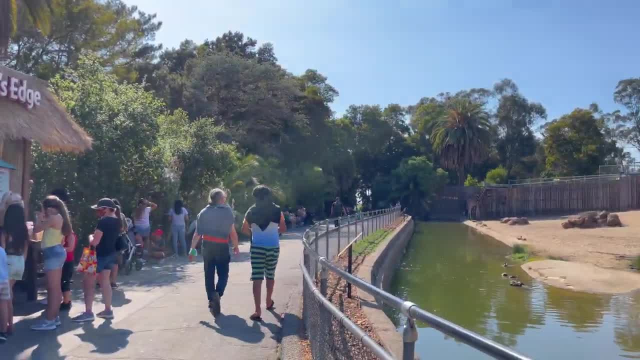 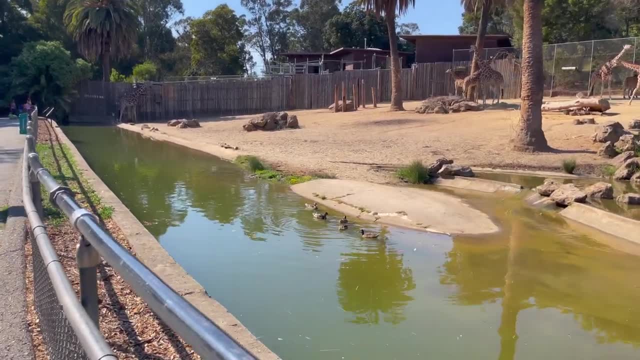 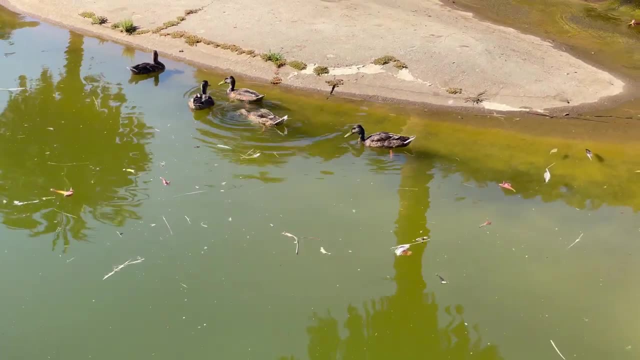 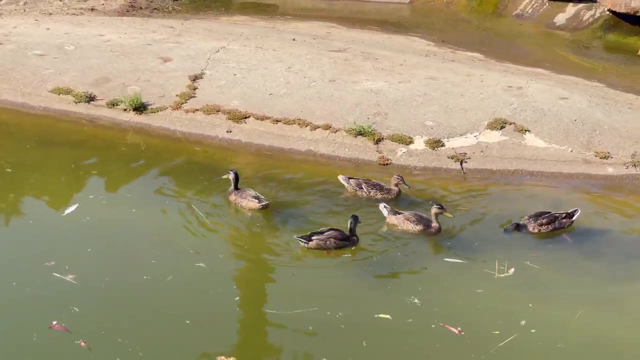 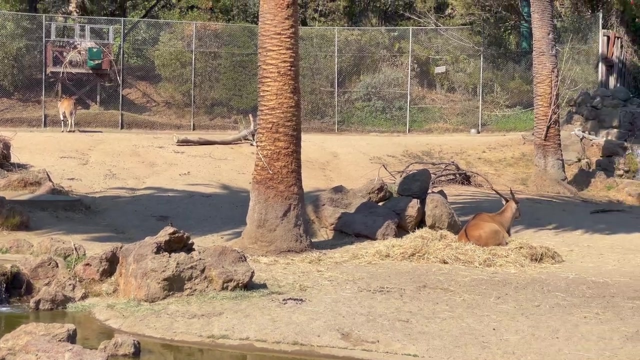 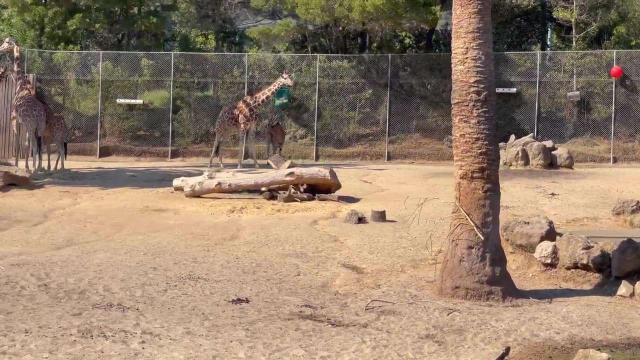 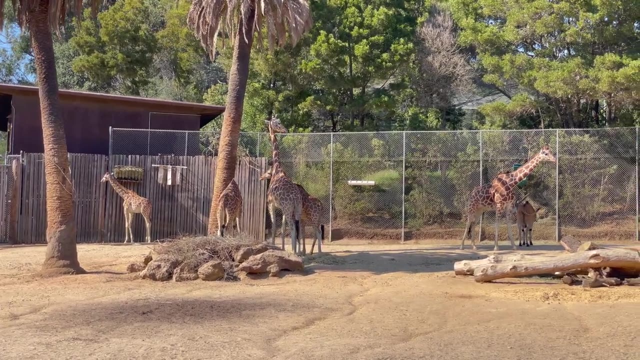 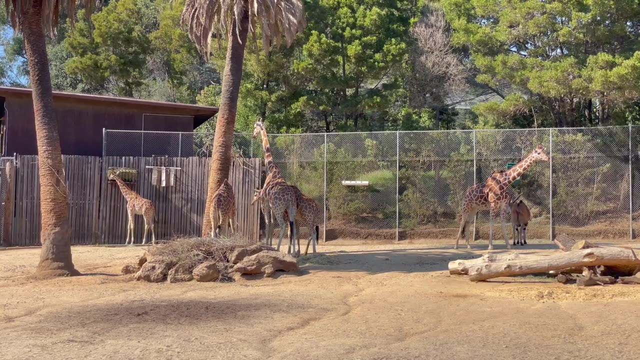 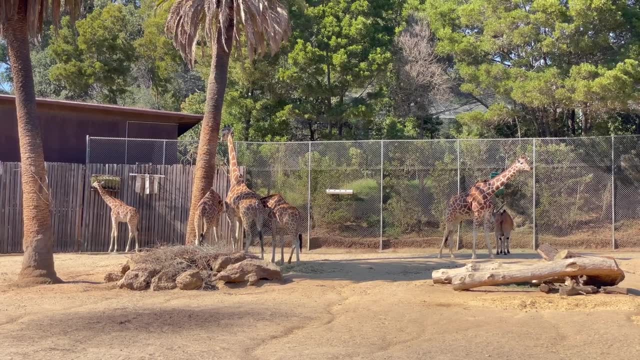 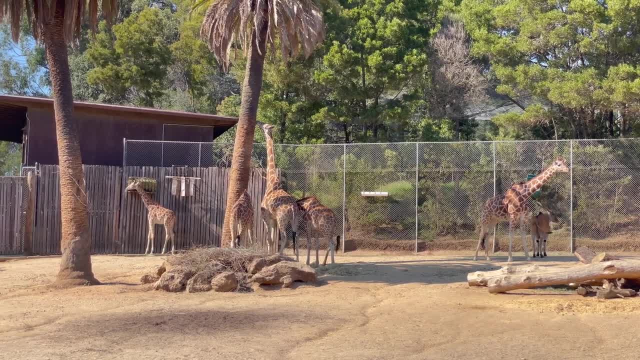 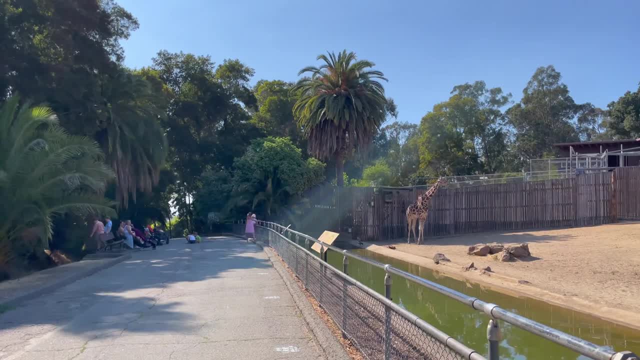 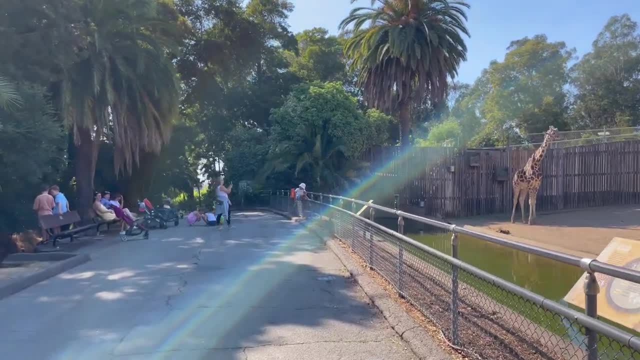 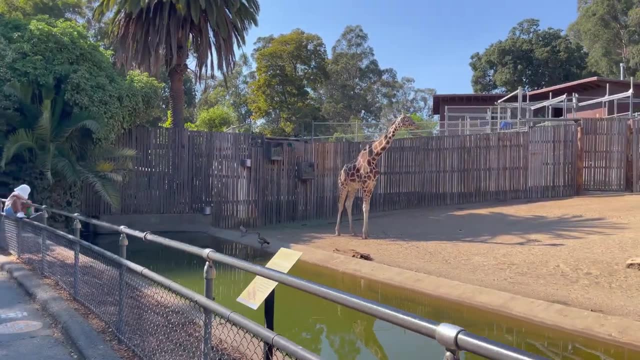 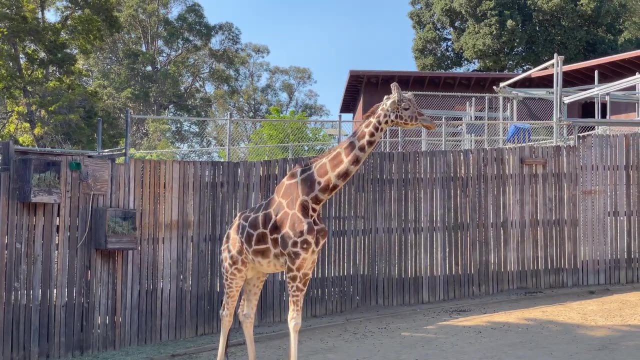 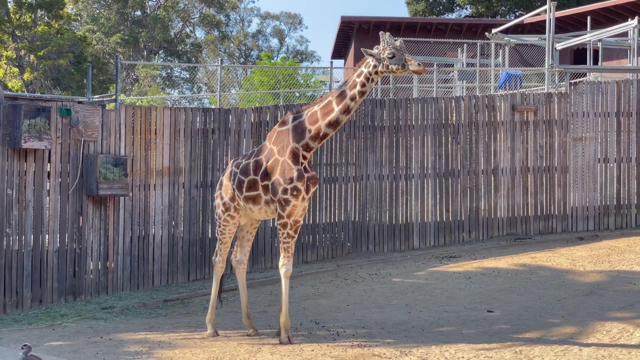 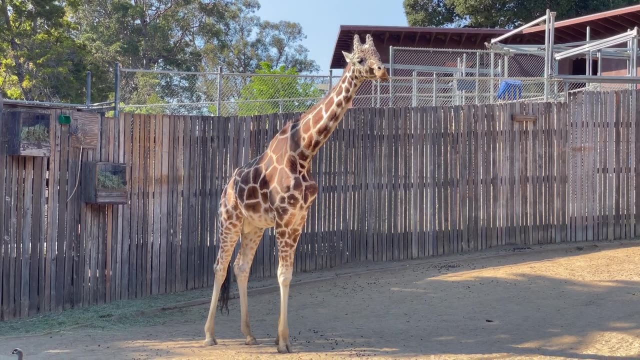 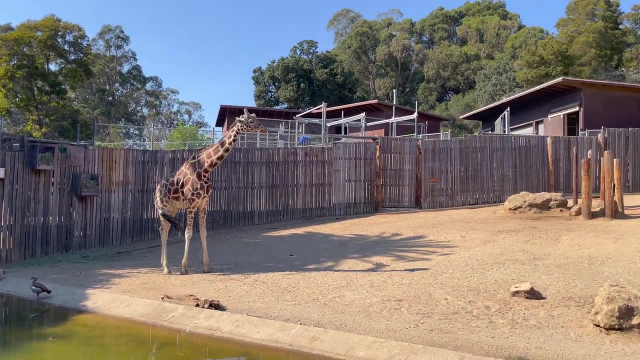 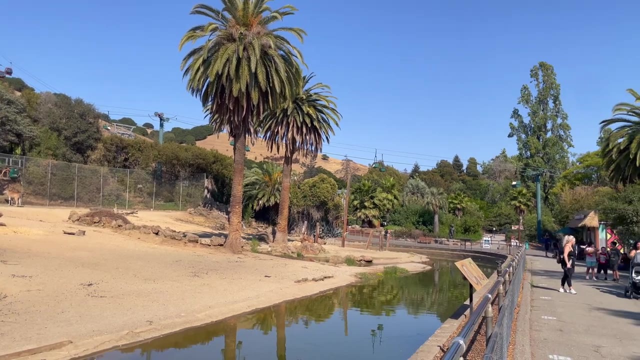 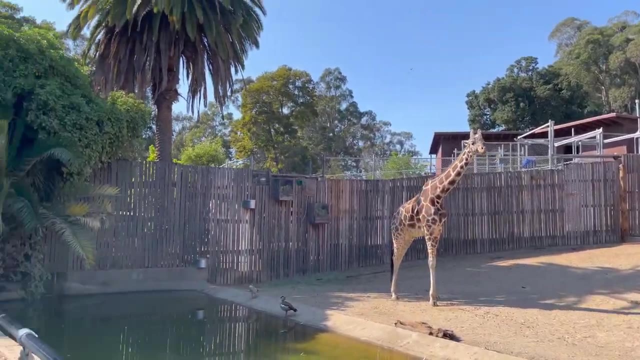 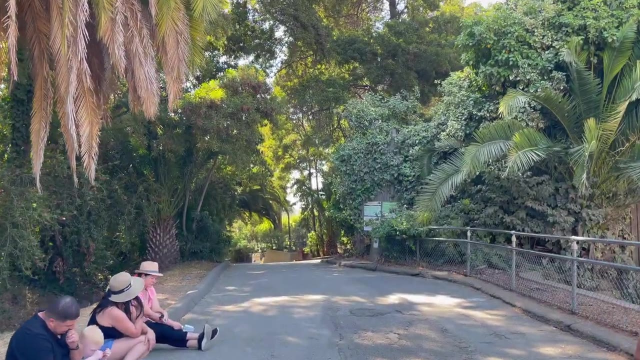 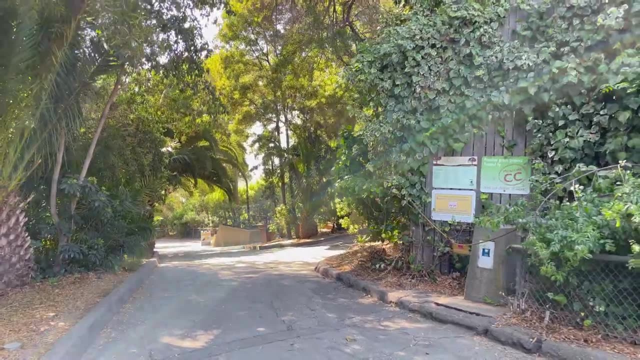 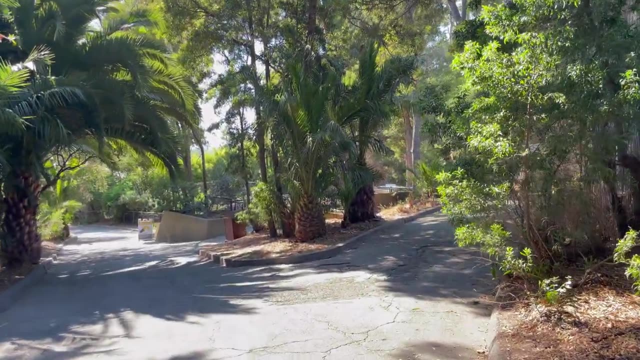 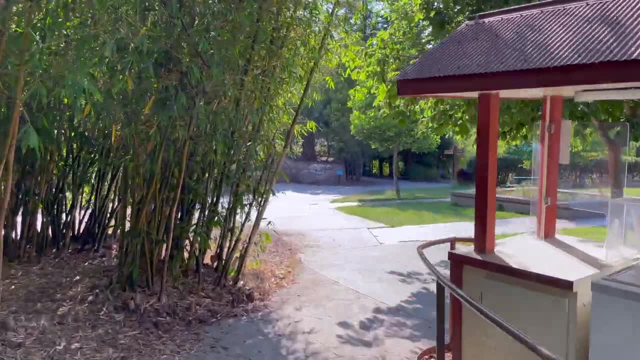 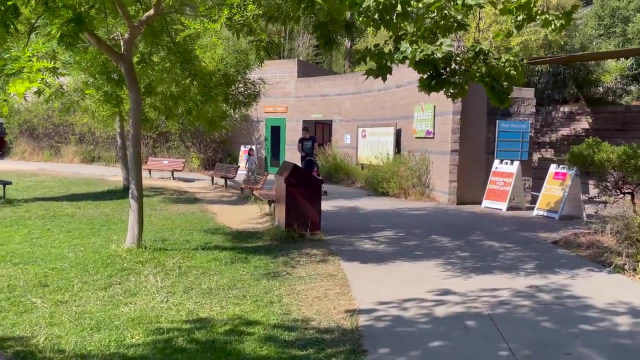 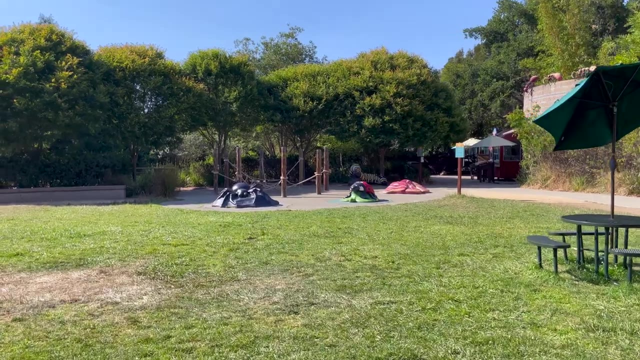 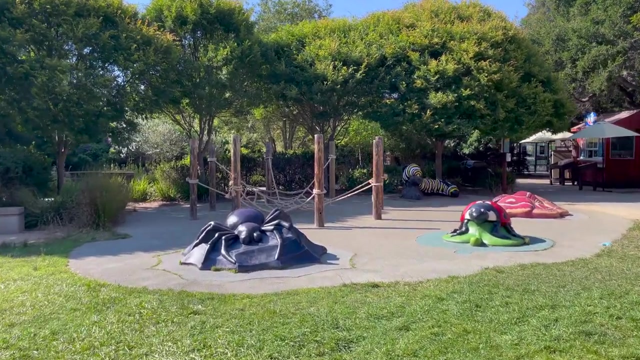 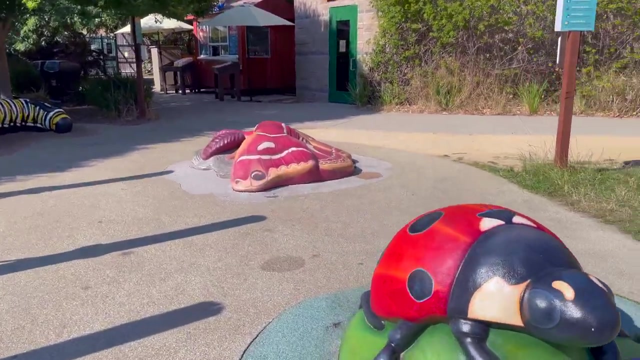 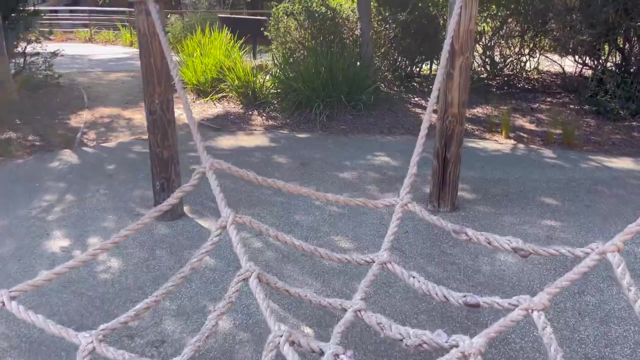 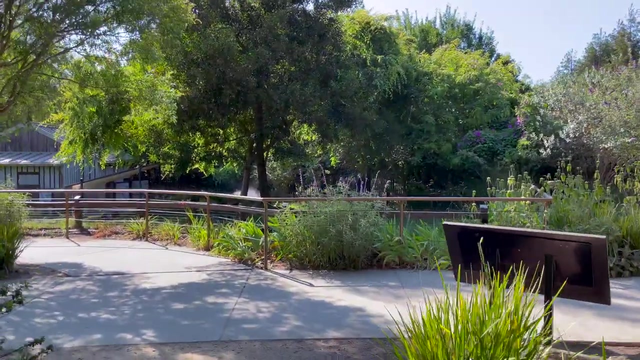 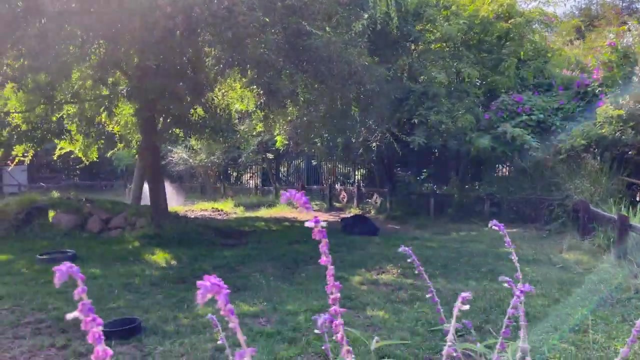 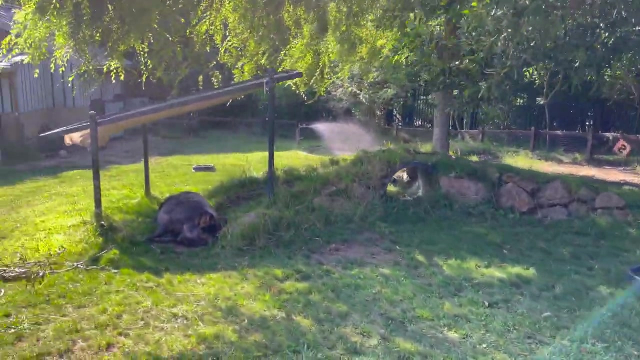 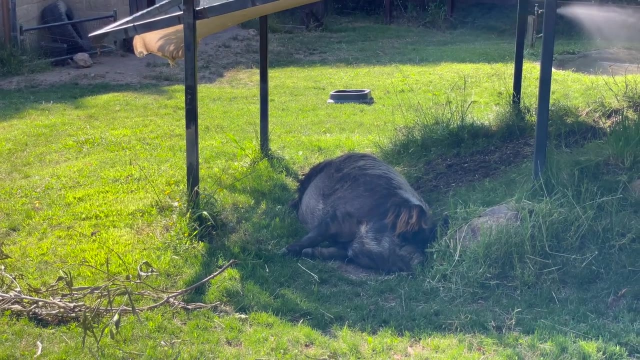 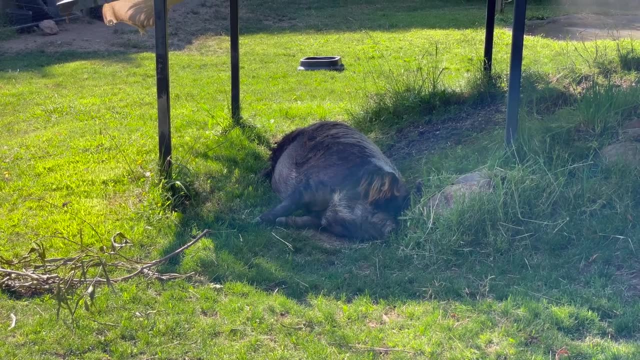 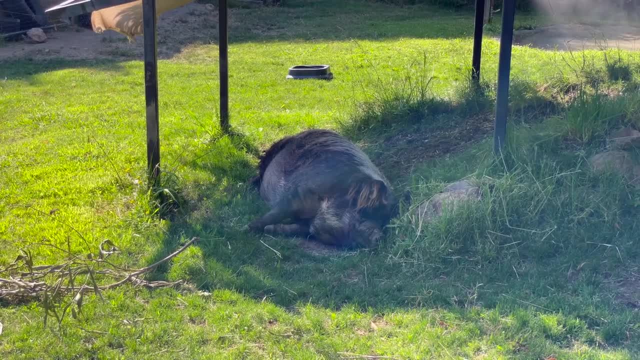 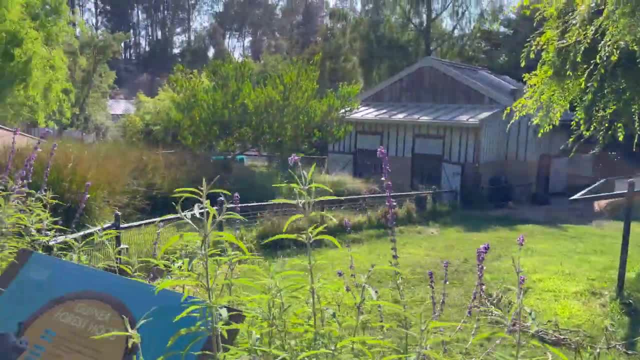 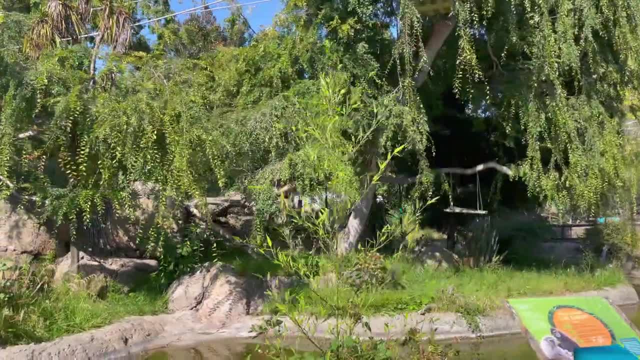 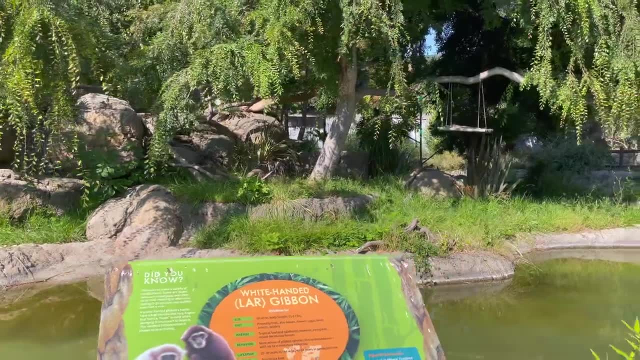 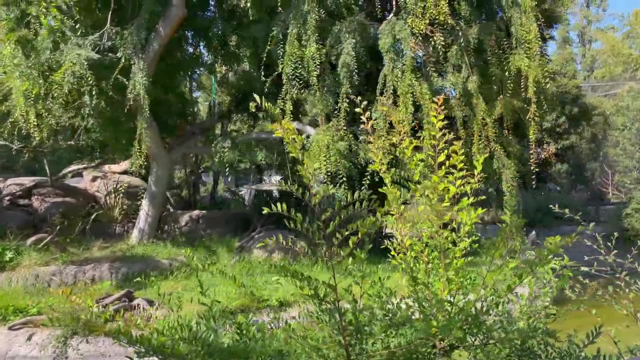 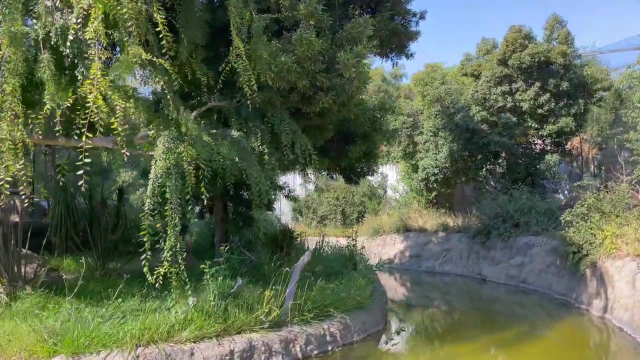 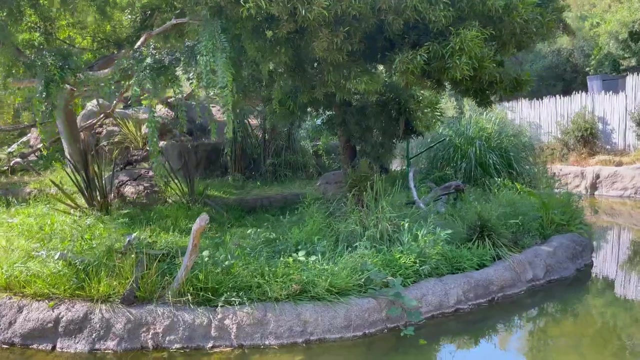 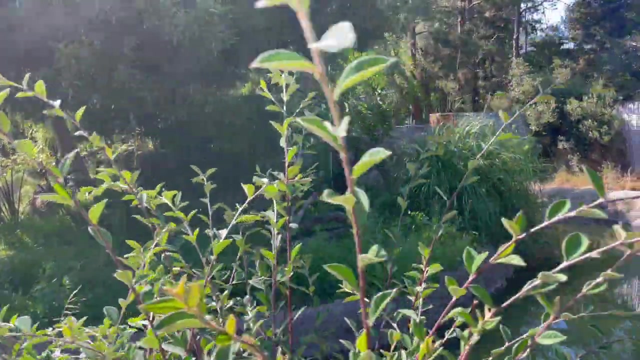 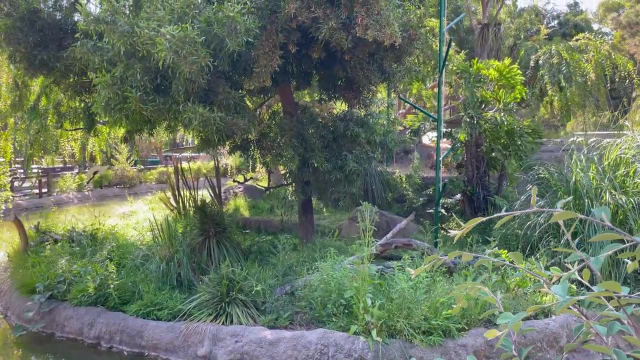 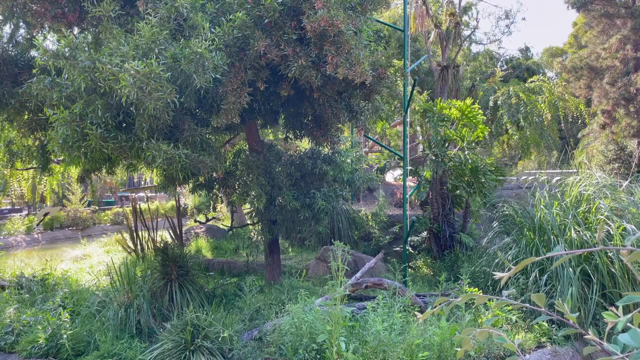 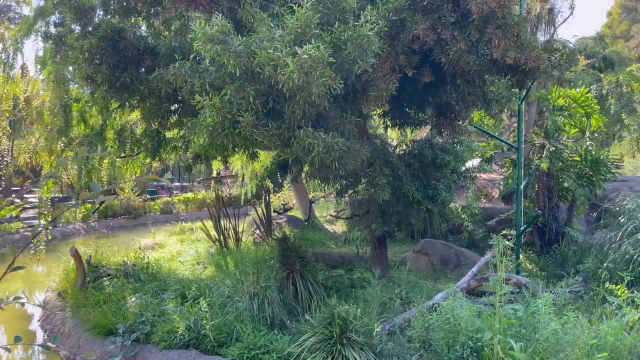 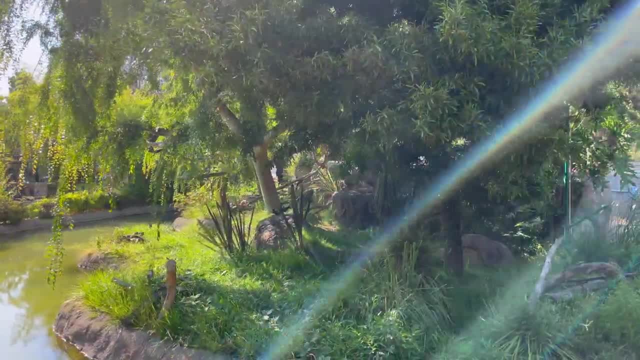 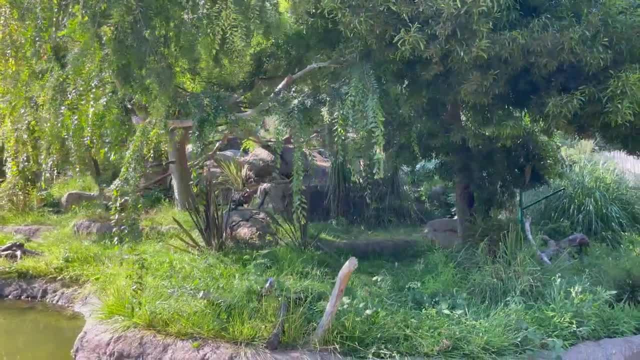 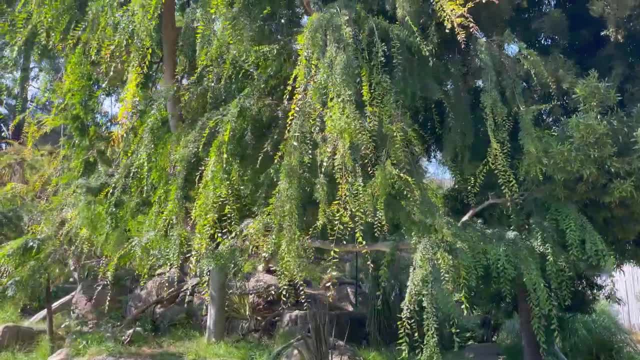 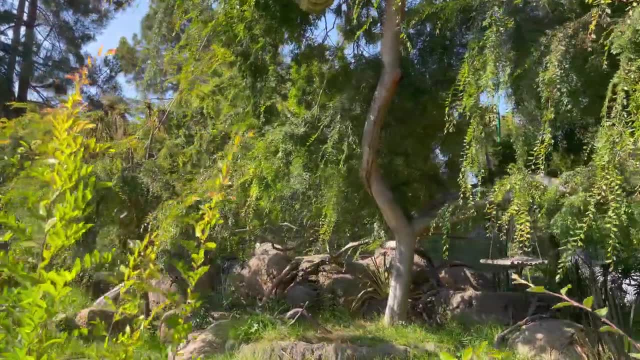 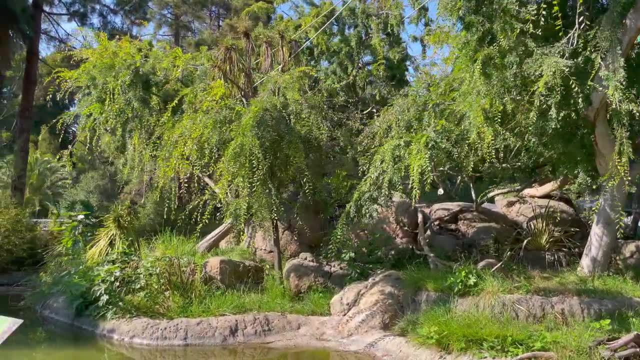 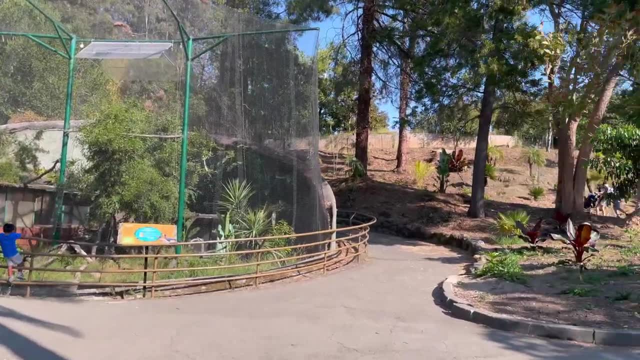 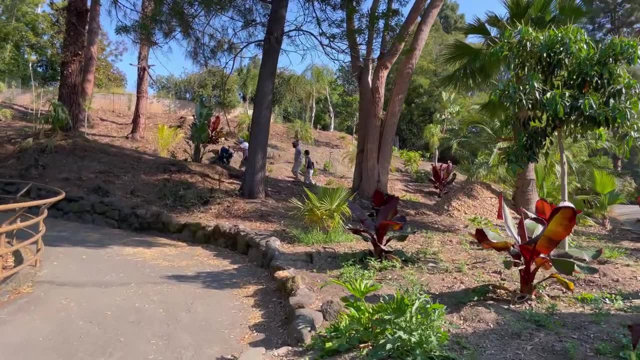 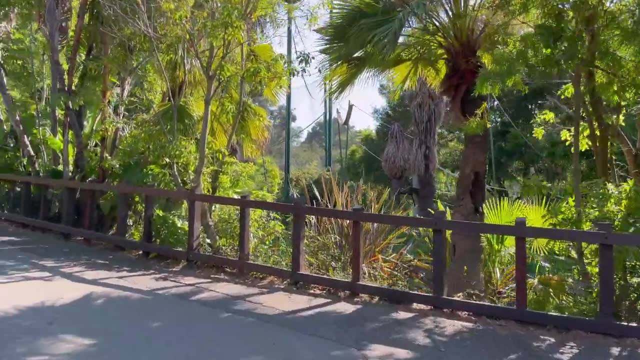 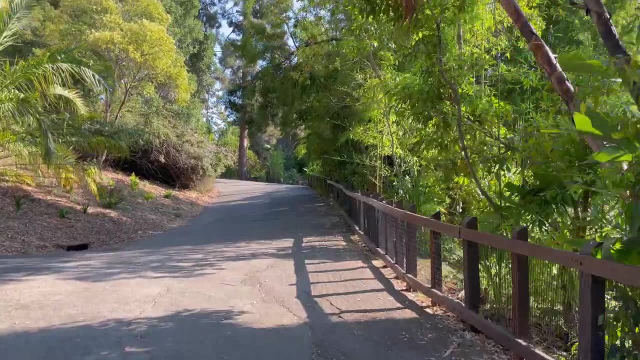 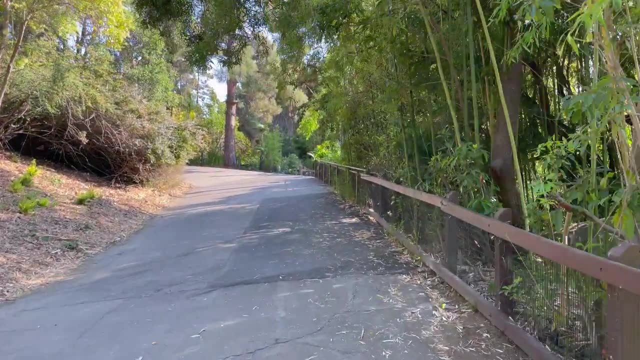 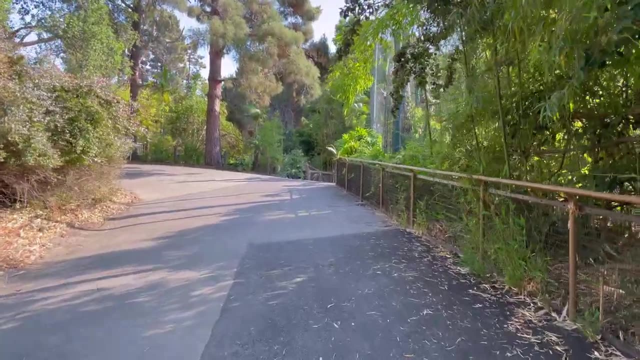 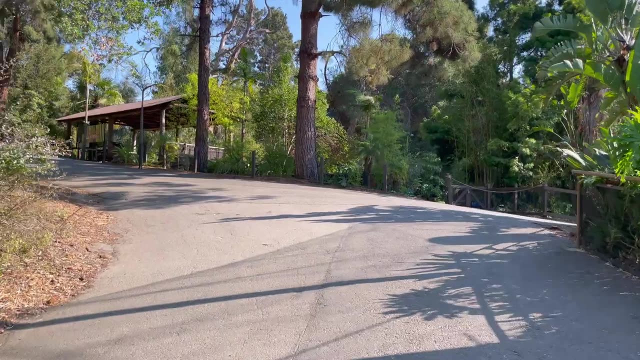 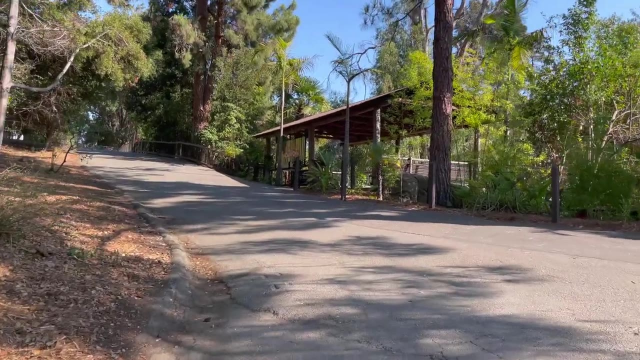 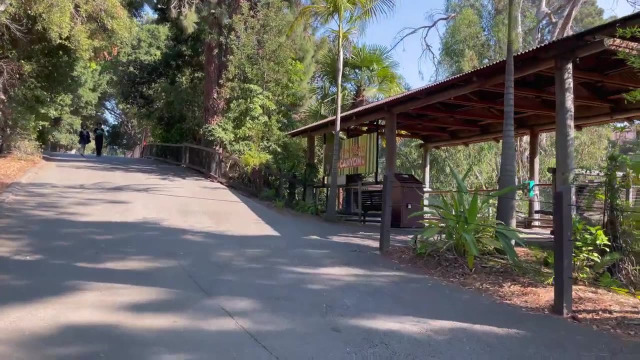 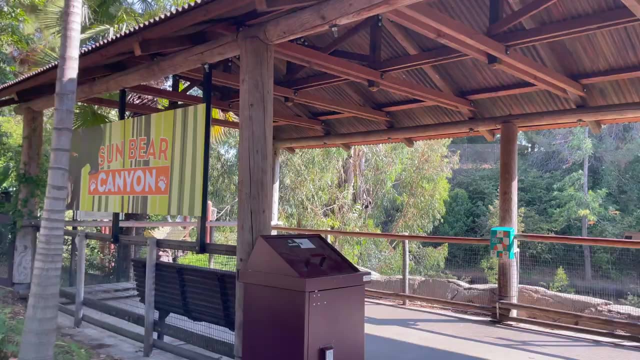 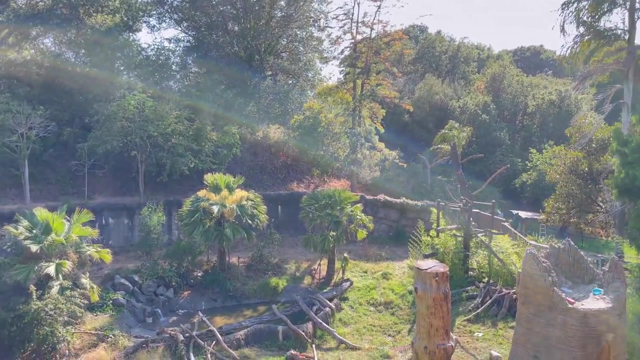 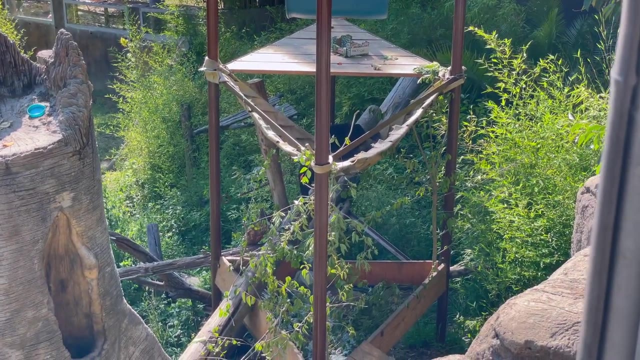 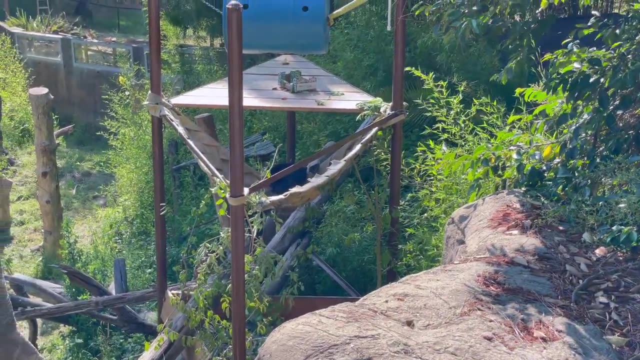 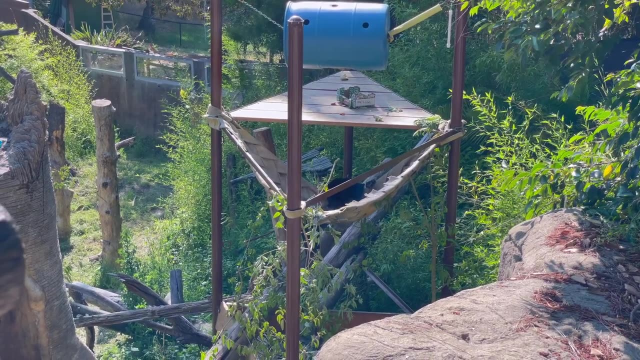 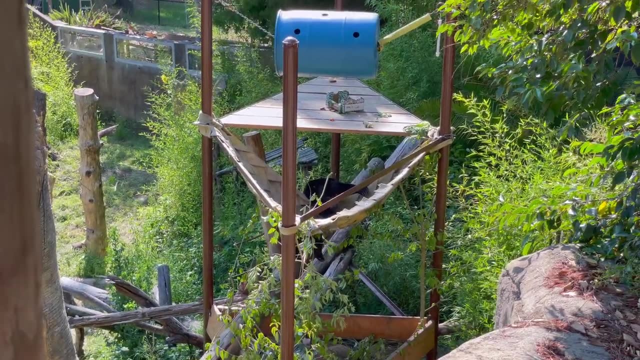 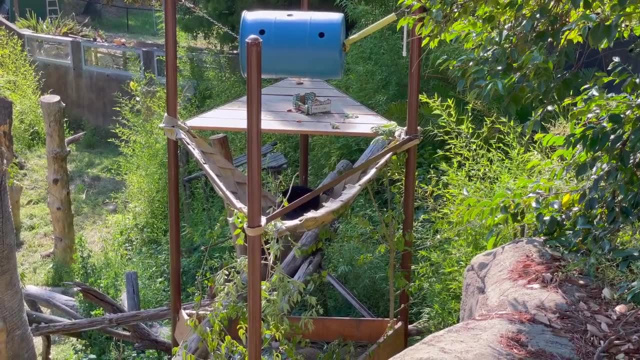 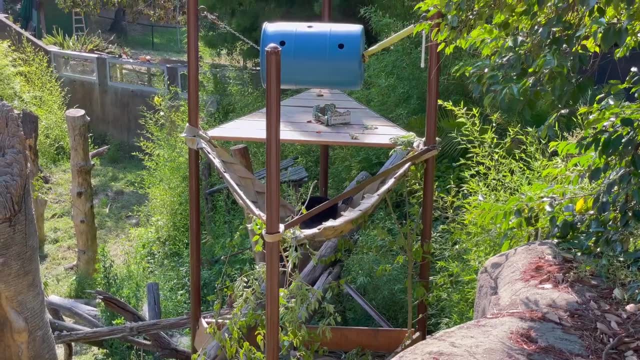 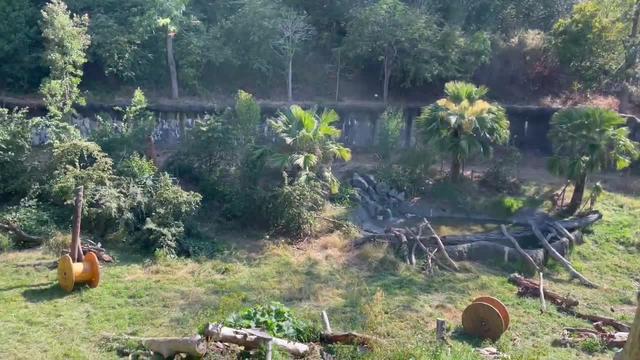 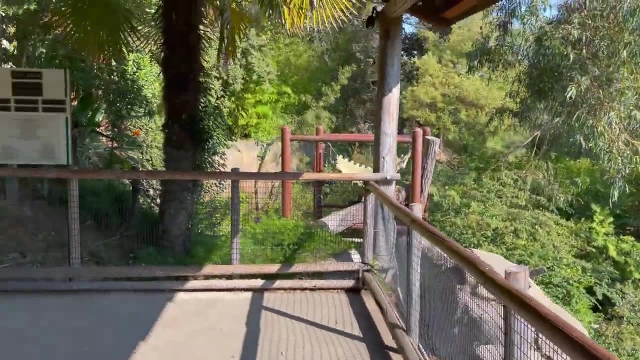 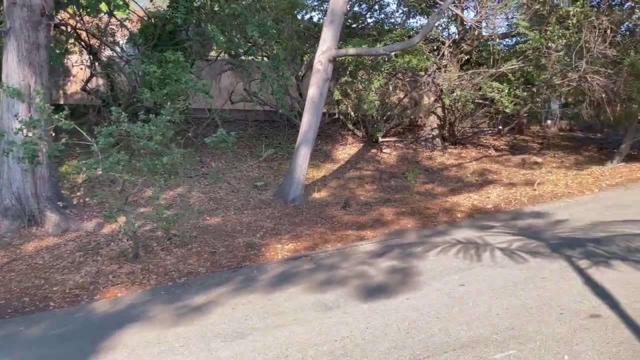 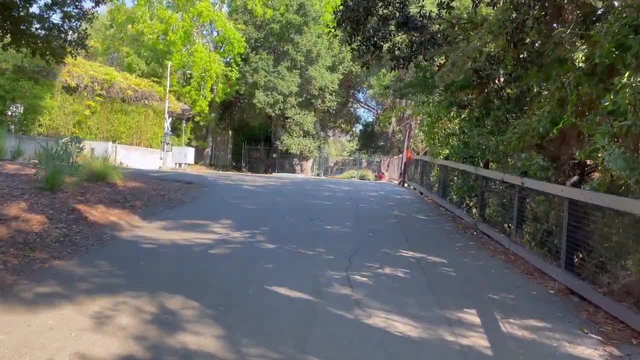 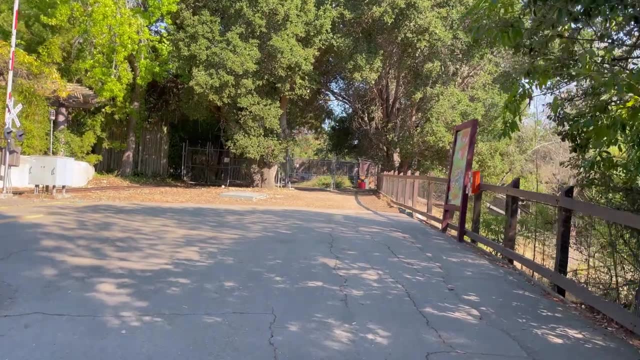 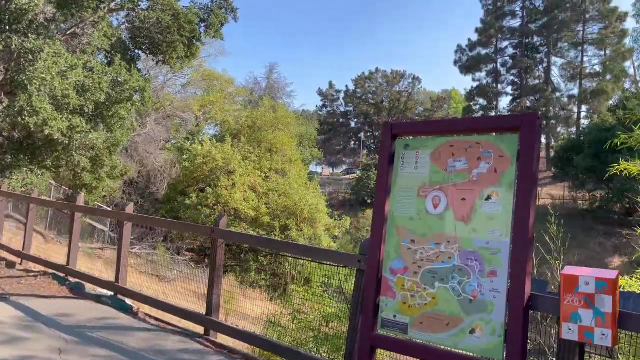 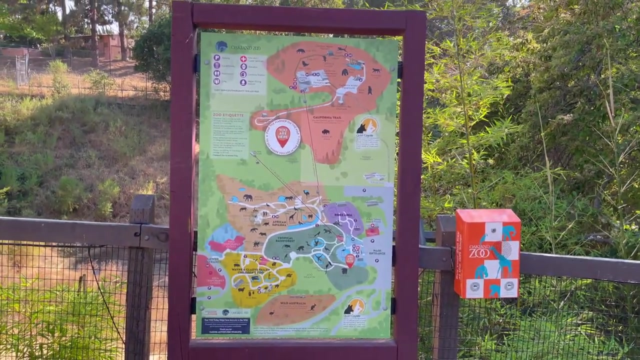 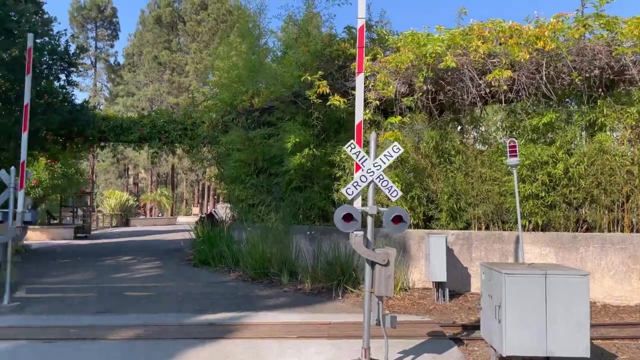 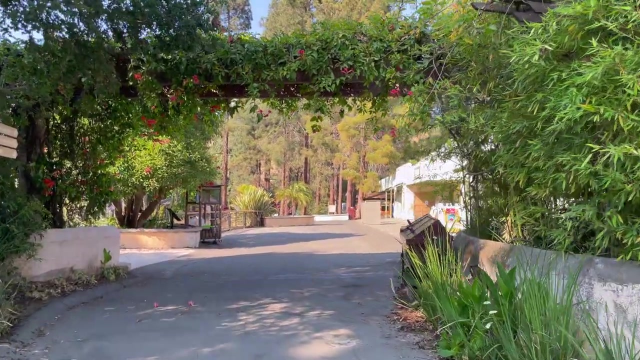 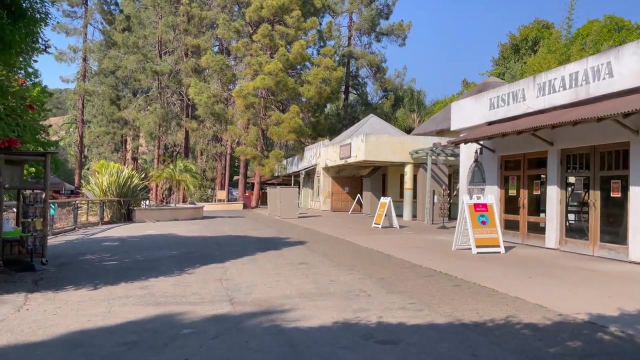 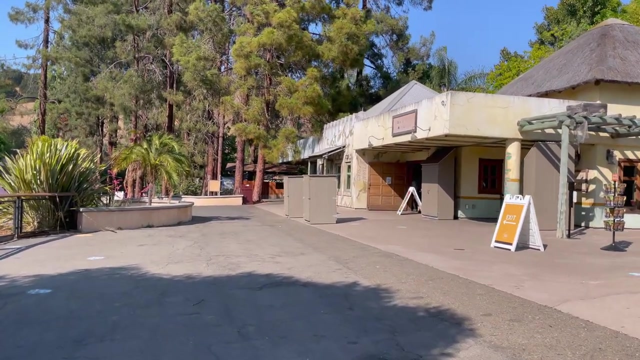 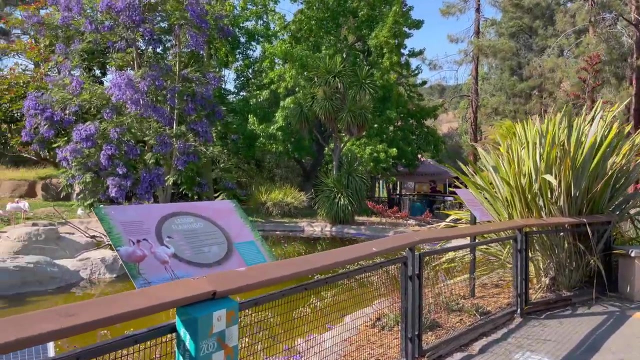 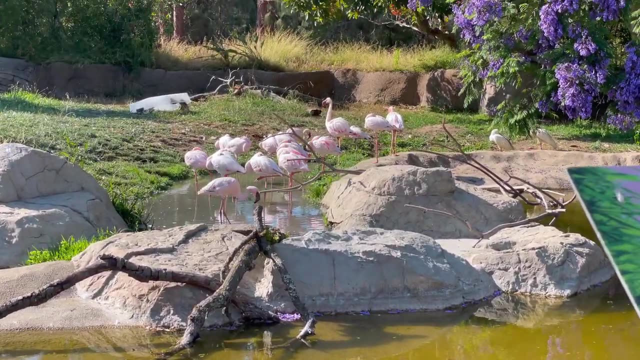 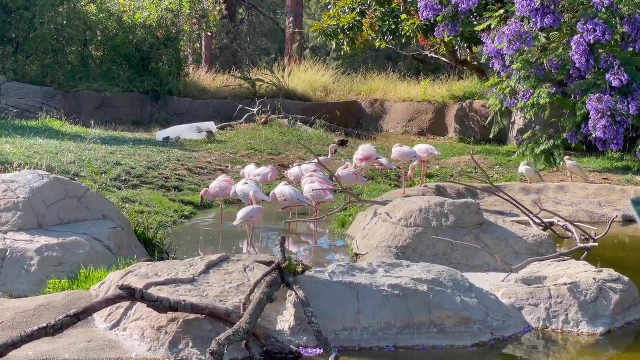 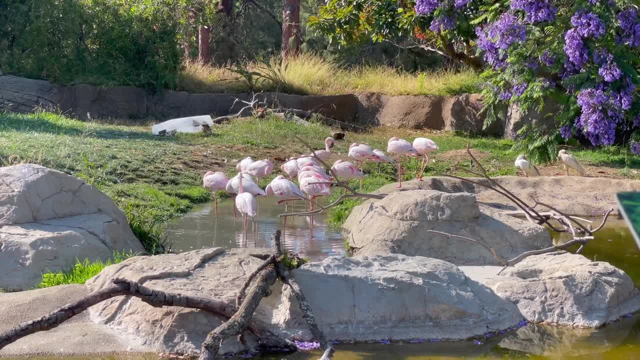 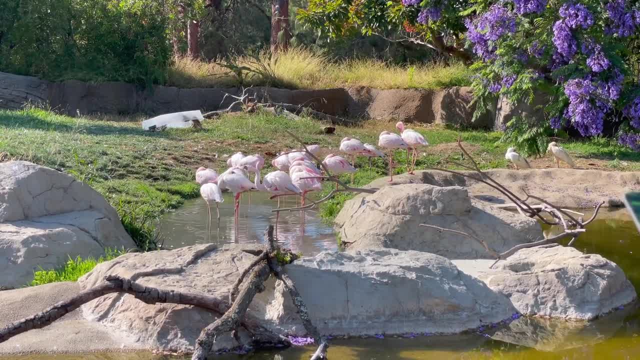 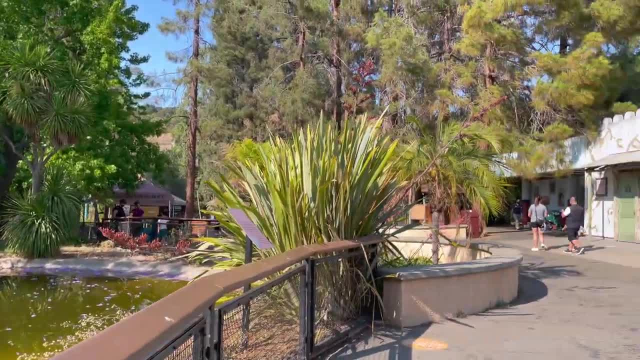 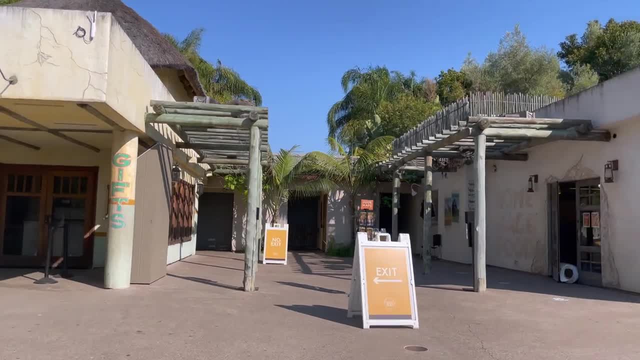 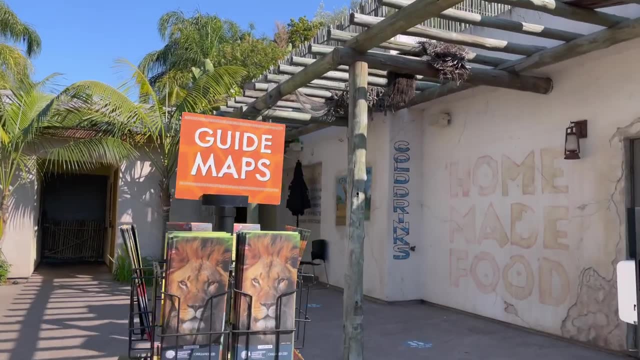 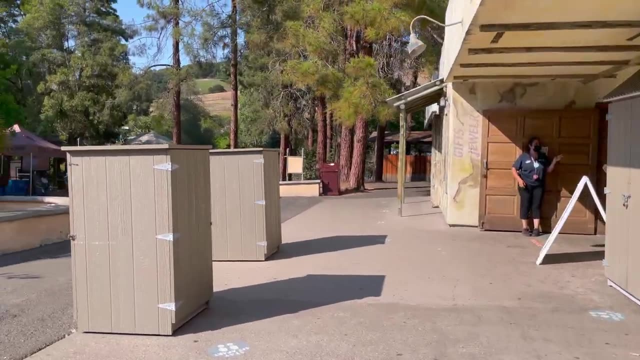 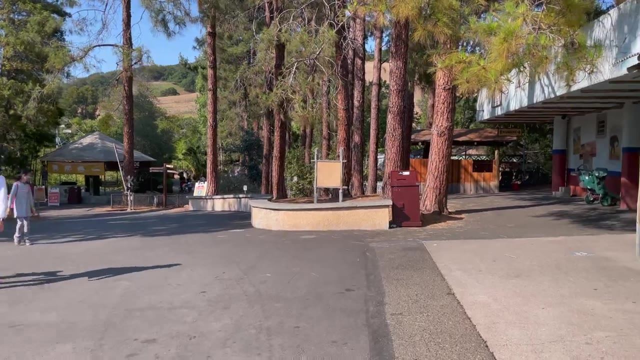 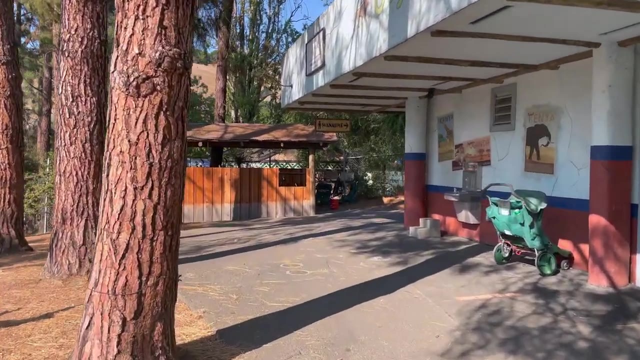 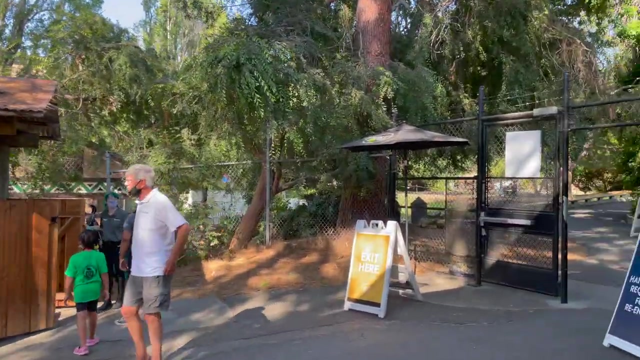 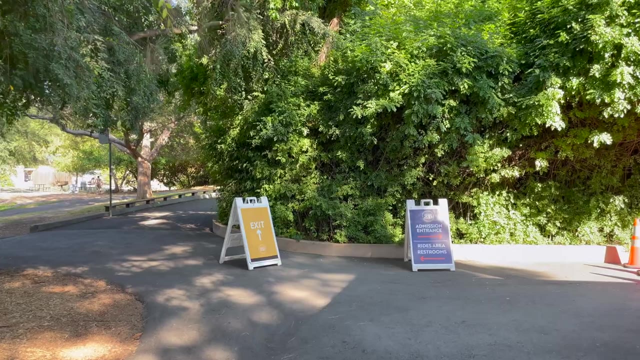 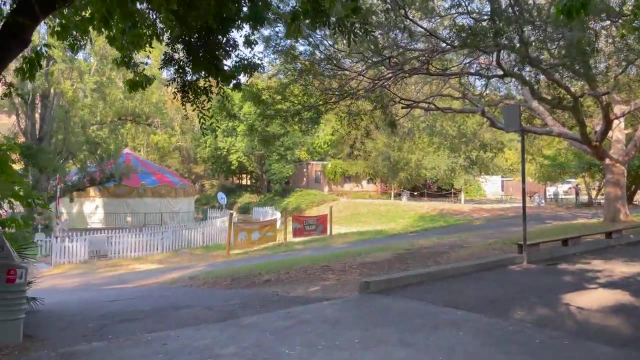 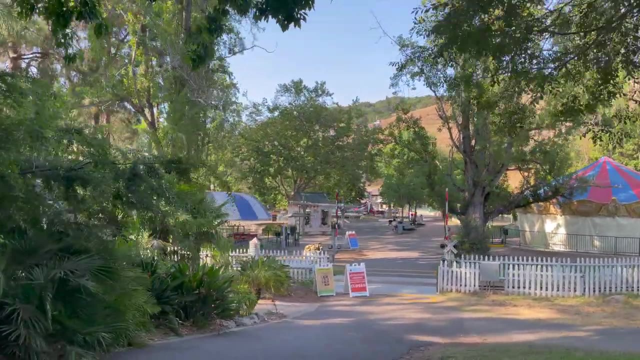 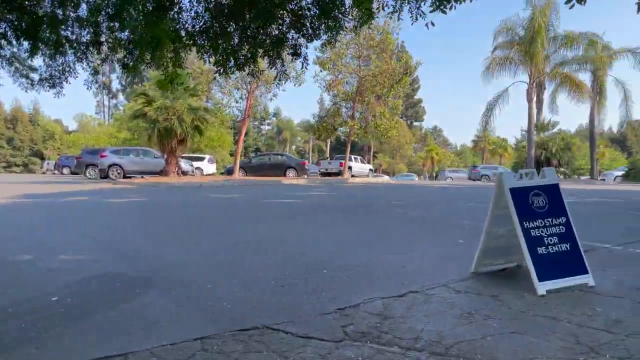 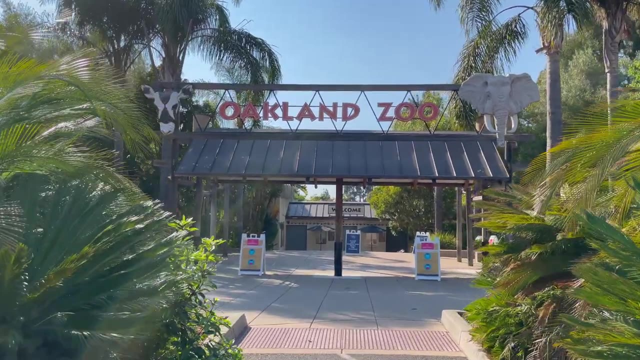 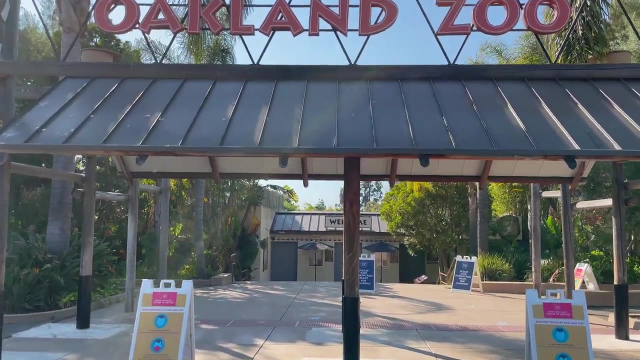 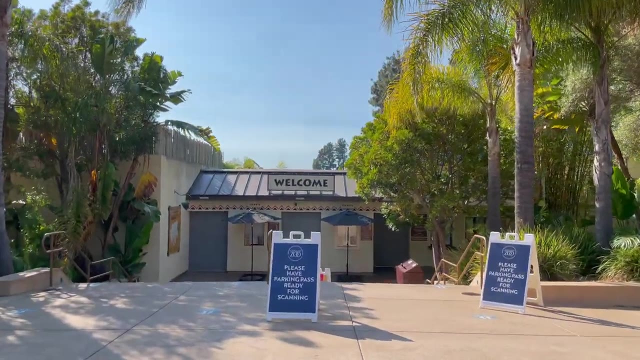 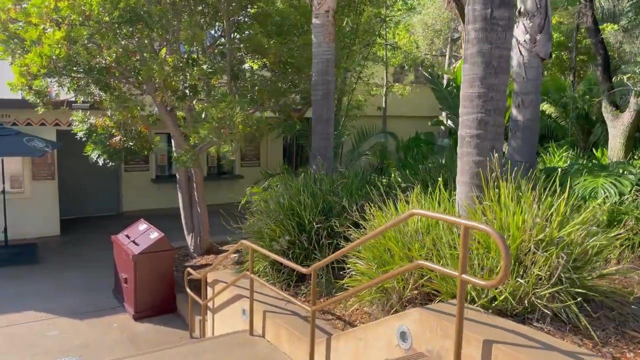 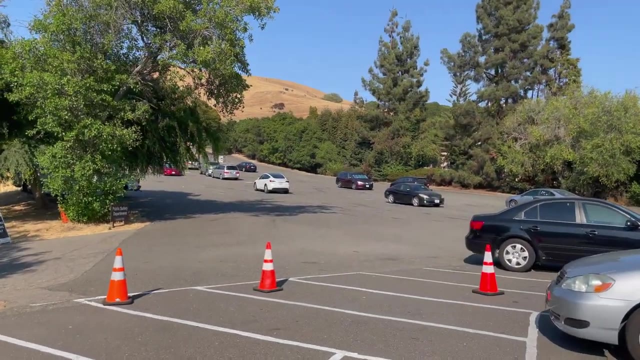